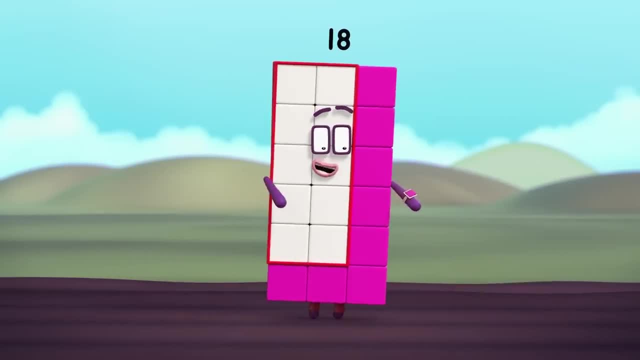 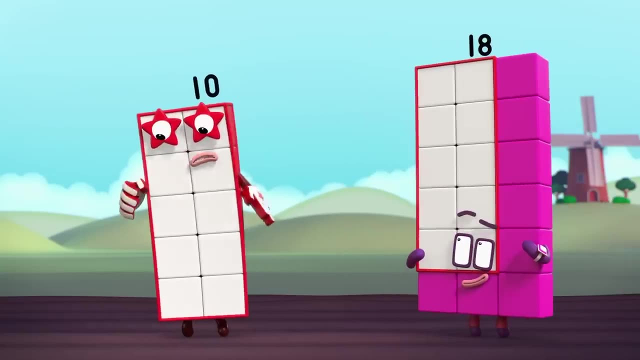 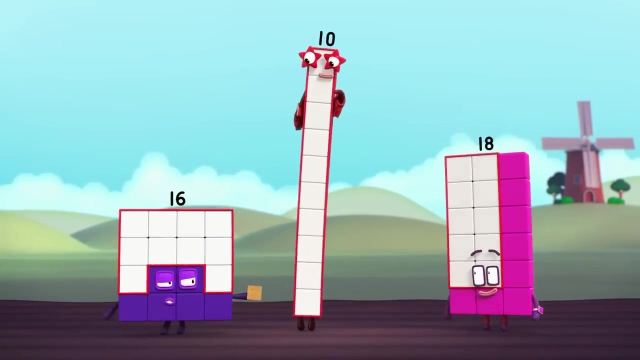 eighteen. Slow enough for you. I'm just adding three. lots of times. The trick is to know how many times. Try it. Ten Um, All right, my friend. I've come to pan some square potatoes. Imagine the chips. 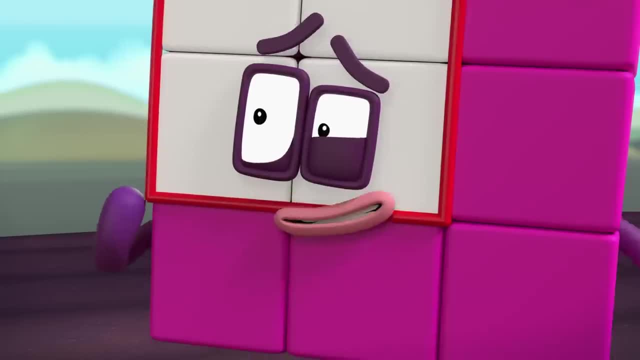 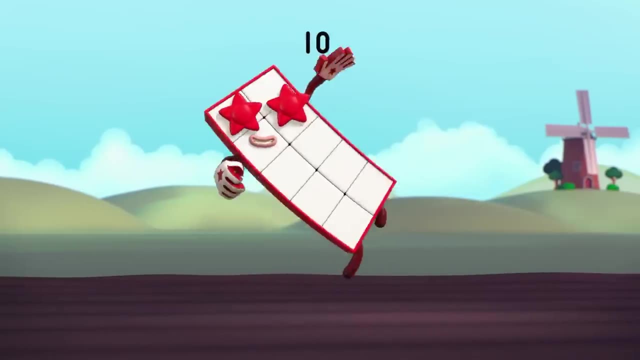 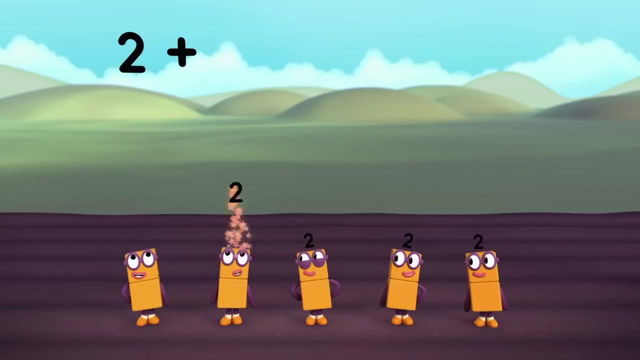 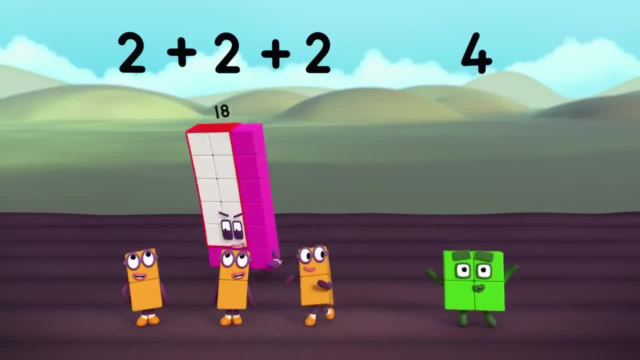 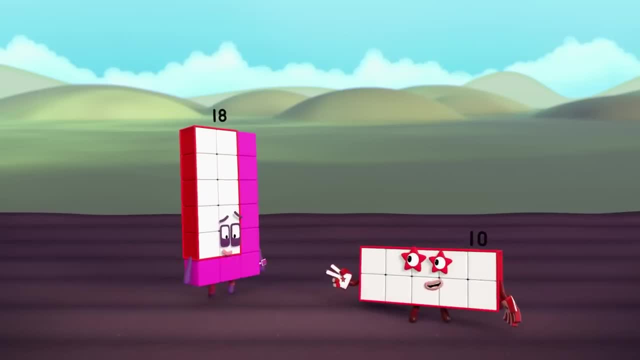 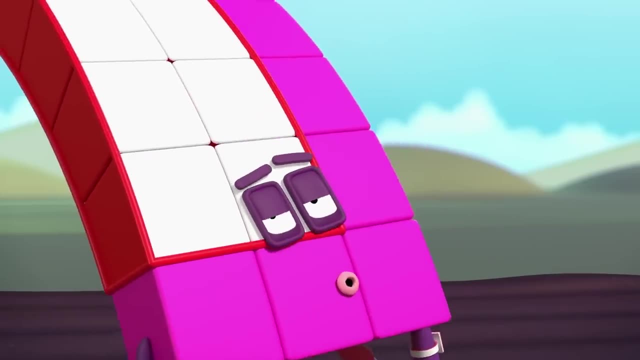 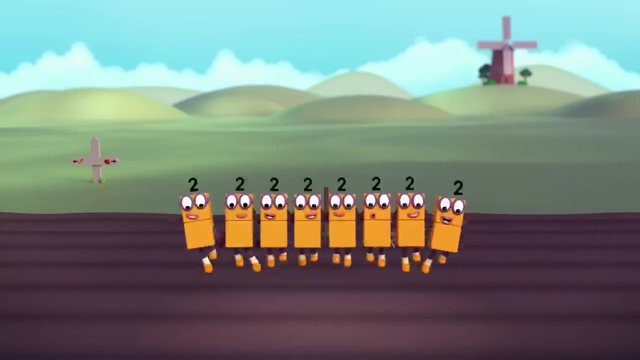 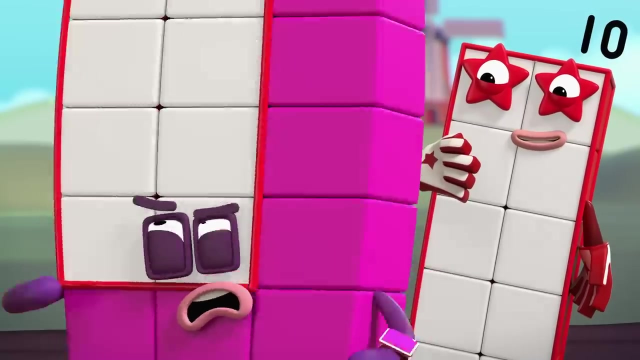 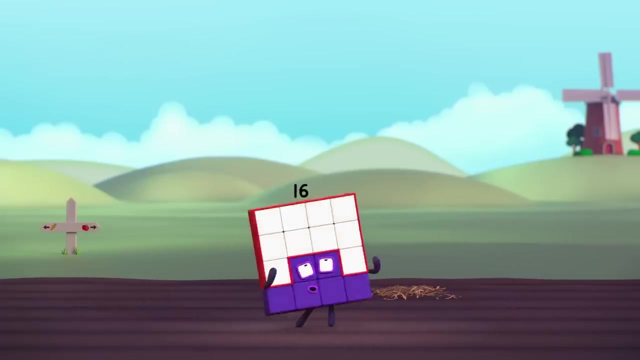 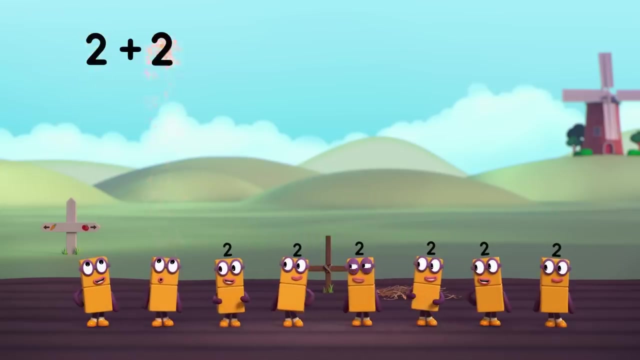 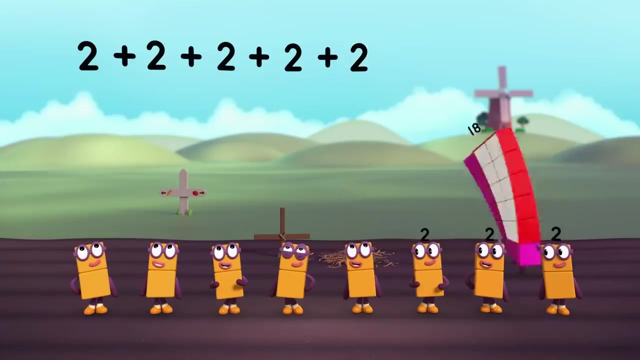 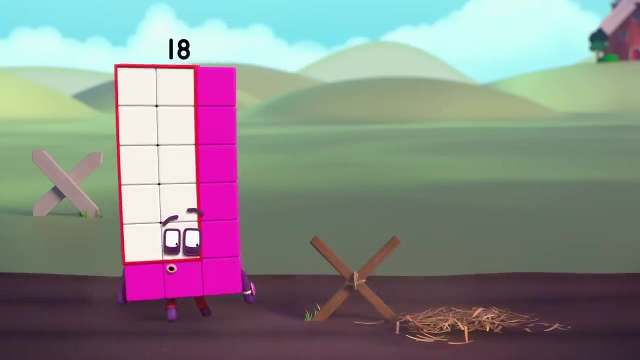 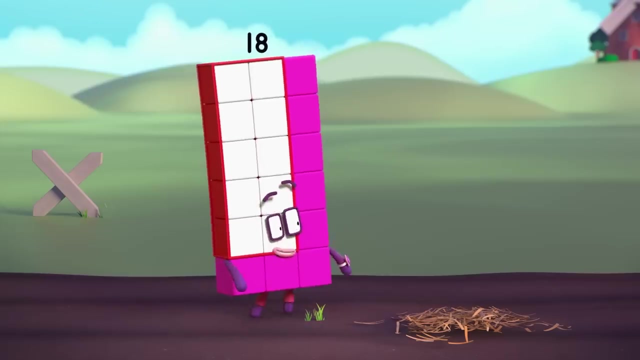 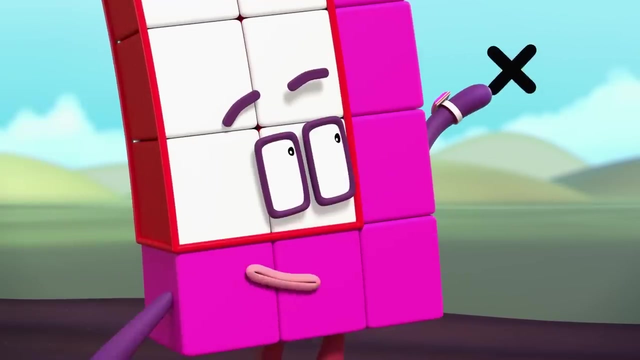 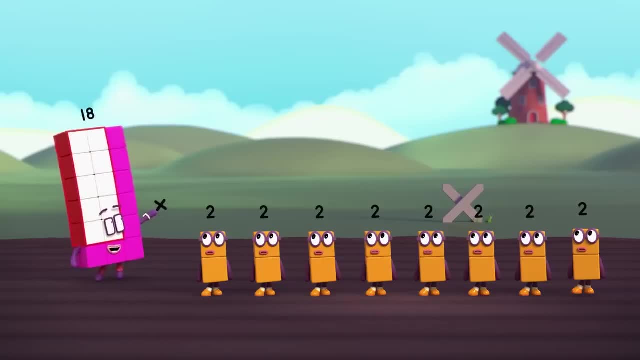 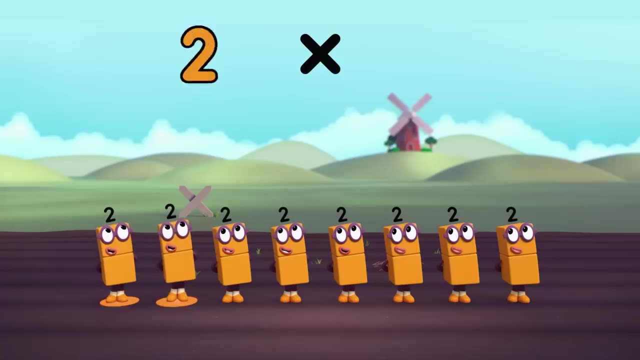 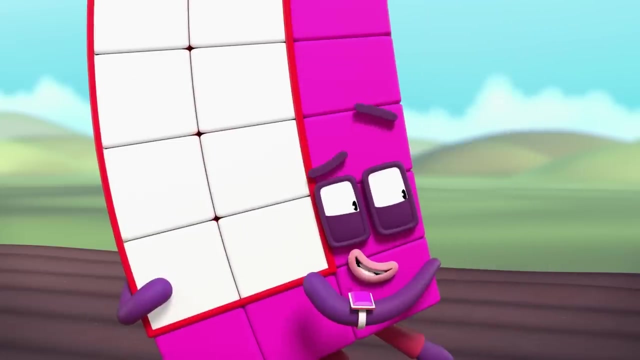 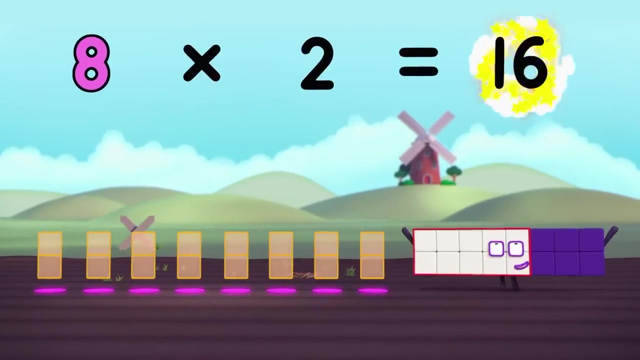 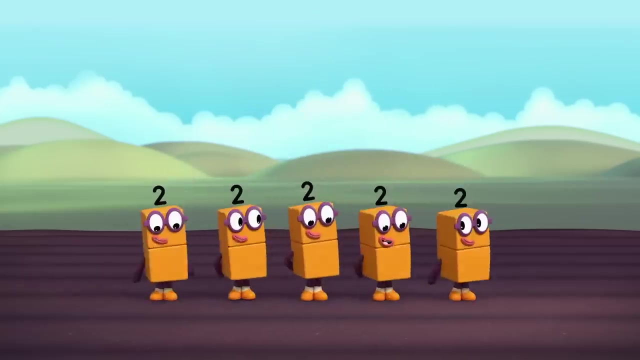 Sign. I can use it to add something lots of times Super quickly. so how many twos are we adding one? Four, five, six, seven, eight, and remind me what Eight. lots of two on your marks. get there. Then go again on your marks. Two equals. 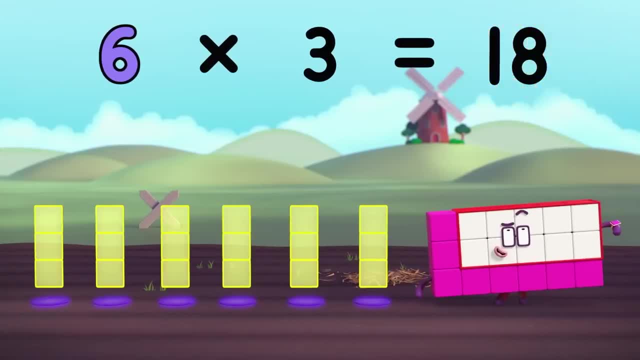 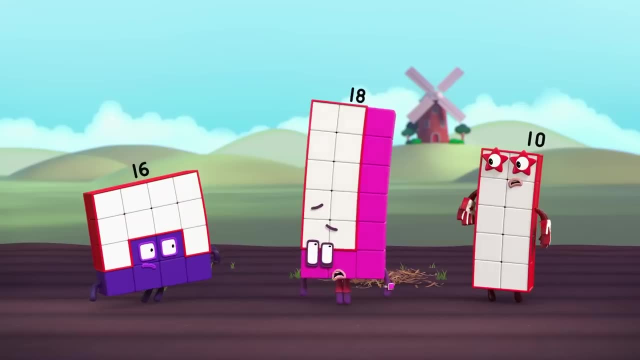 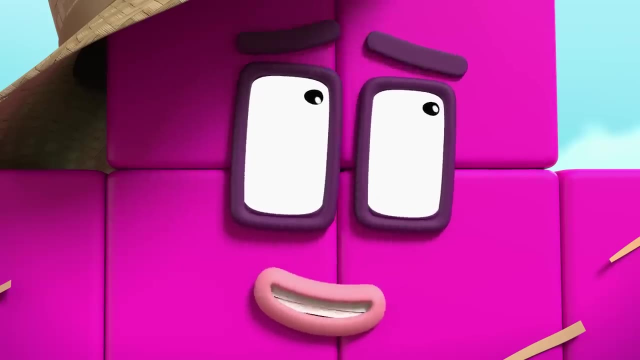 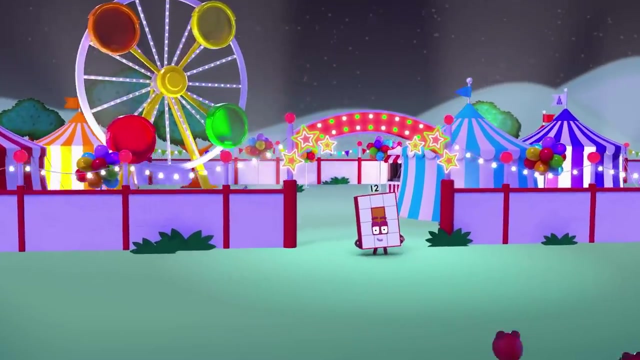 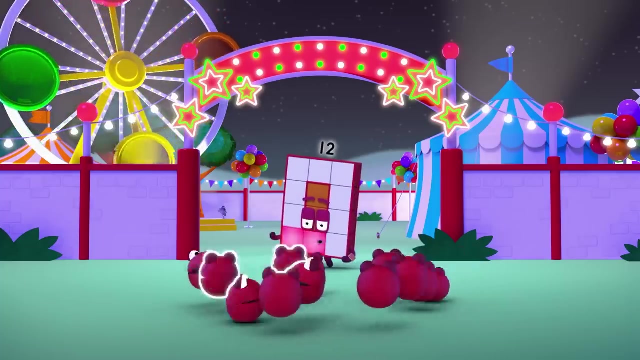 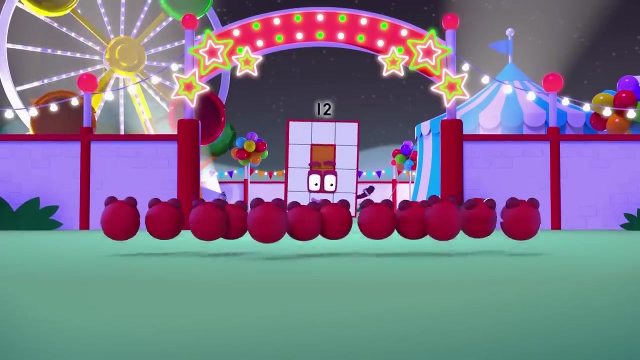 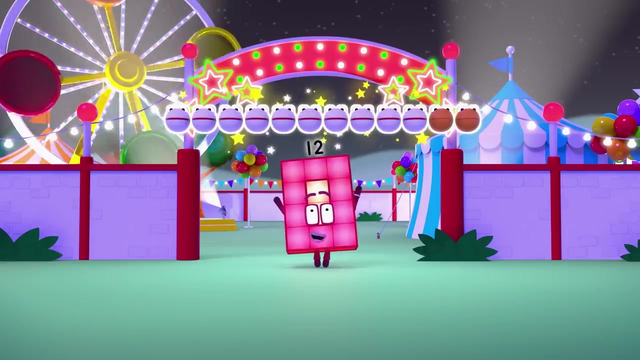 Three equals. This makes up for breaking some silly old Scarecrow. 18. I can't see any 18, just this good old Scarecrow. Oh, Welcome to the fun times. back is everyone here. One, two come here. One, two, three, four, five, six, seven, eight, nine, ten, eleven, twelve, twelve, number blobs, good. 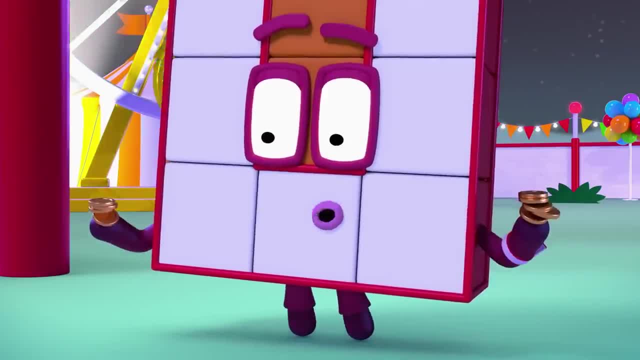 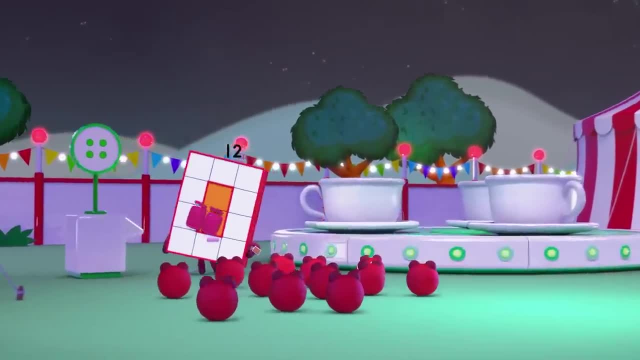 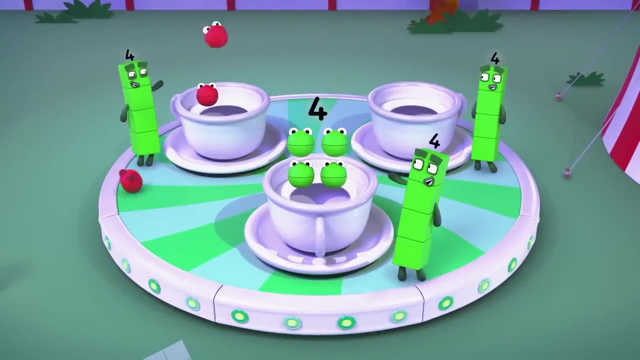 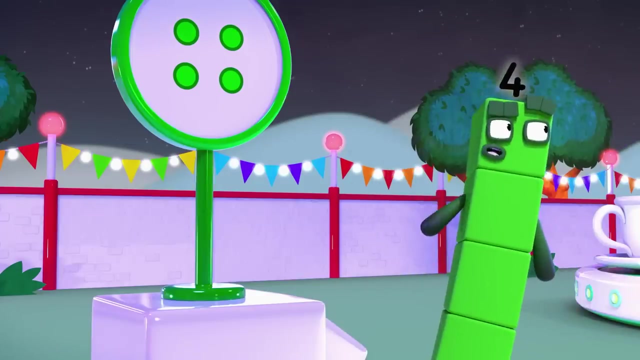 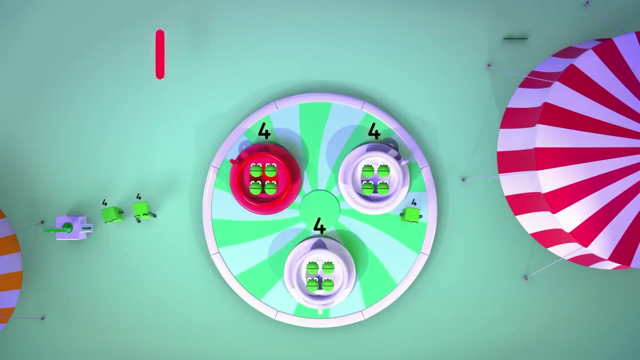 I've got lots of right tokens. What would you like to? I believe I can. I can The deeper. Don't give up Woop. a good, quiet Good, do I he? I believe him, associate. That's the goal. Anthony I the cé m now Uno Dos. 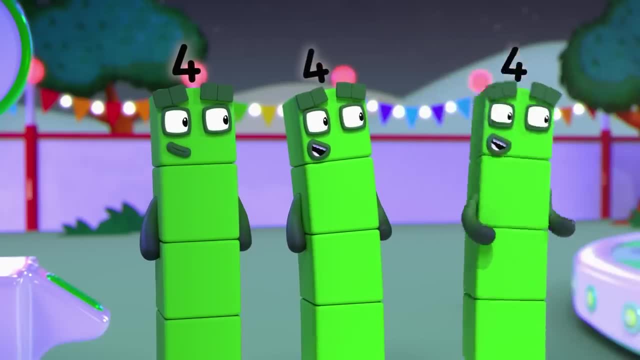 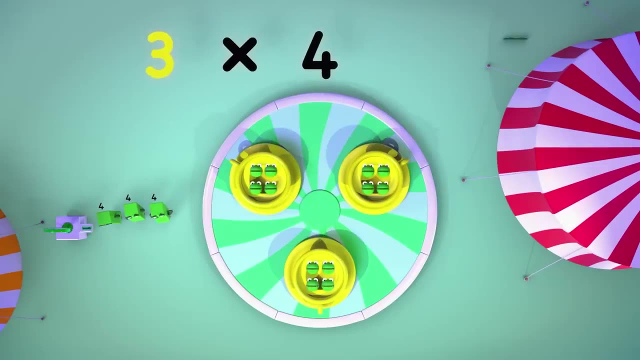 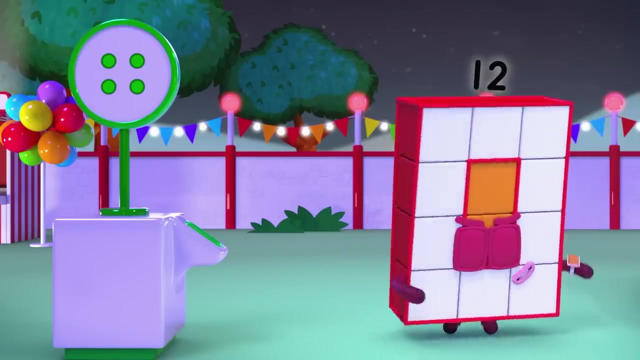 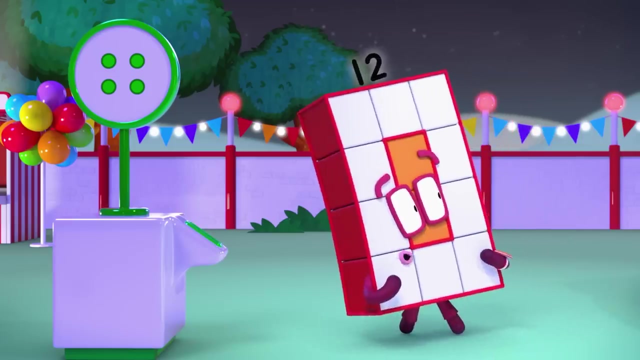 Three cups And how many riders in each cup? Four. So that's three lots of four. Three times four, which is Three times four, equals twelve. Three lots of four is Twelve tokens. And off you go, Watch us spin. three lots of four. Twelve number blocks and not one more. 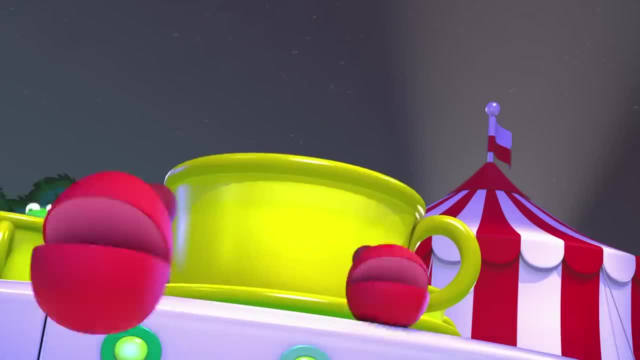 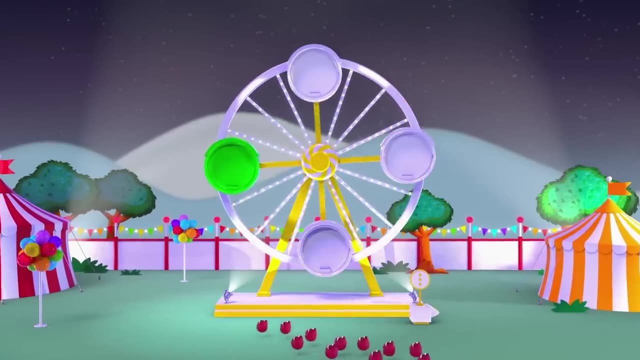 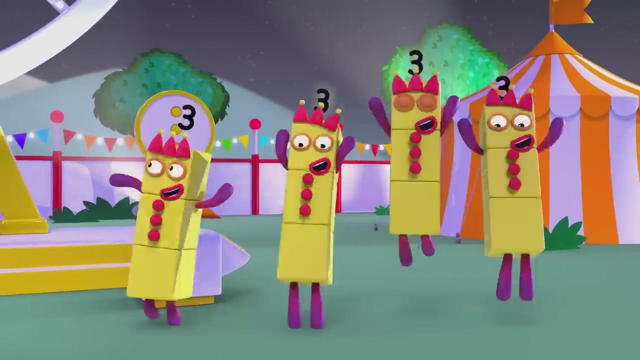 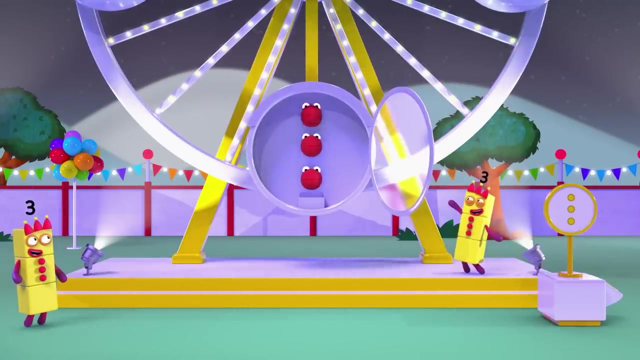 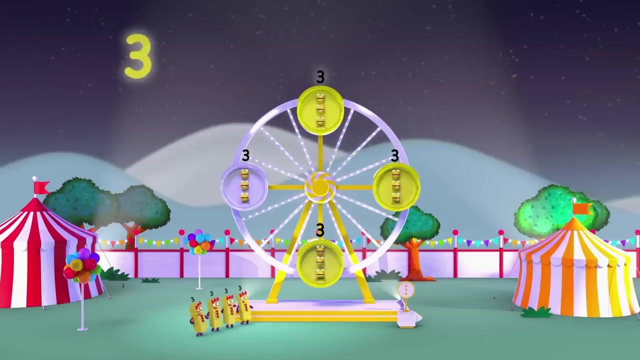 Three. That was fun. So The big wheel, The big wheel, Aha, Looks like three to a carriage this time: Two, Three, Three, Three, Three Time for tokens. How many carriages? One, two, three, four. 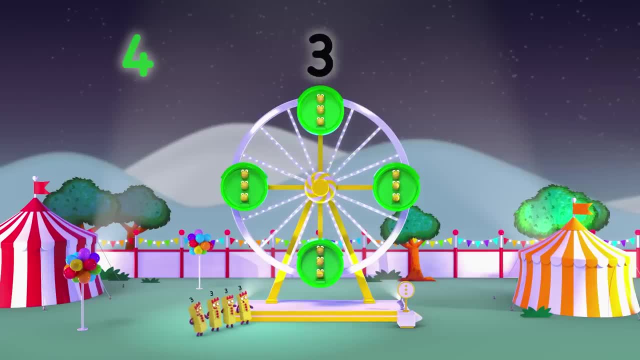 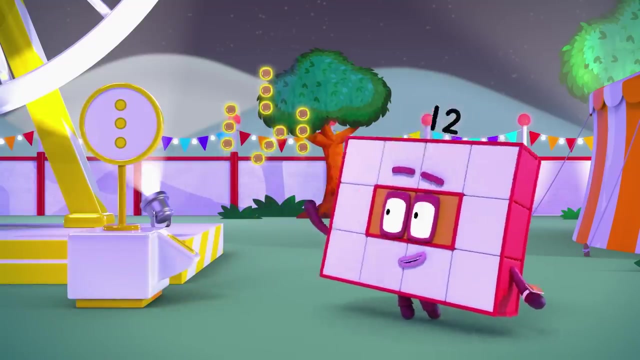 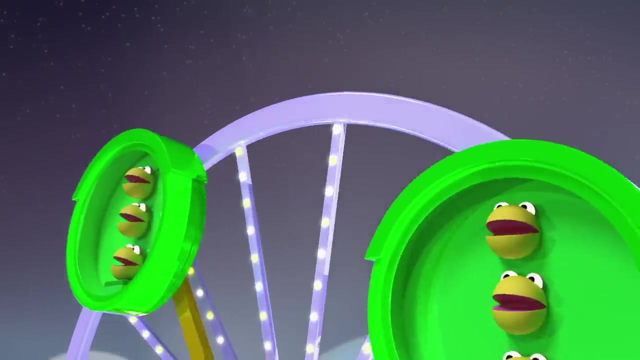 How many in each carriage? Three. So how many tokens do you need? Four times three equals twelve. Three, Three, Twelve tokens, Four, lots of three, Around we go. Four groups of three, Twelve number blocks all going wee. 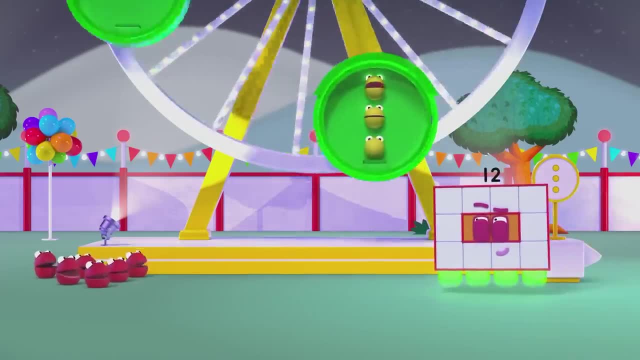 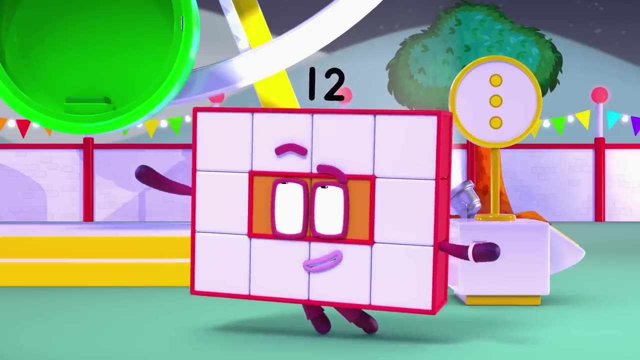 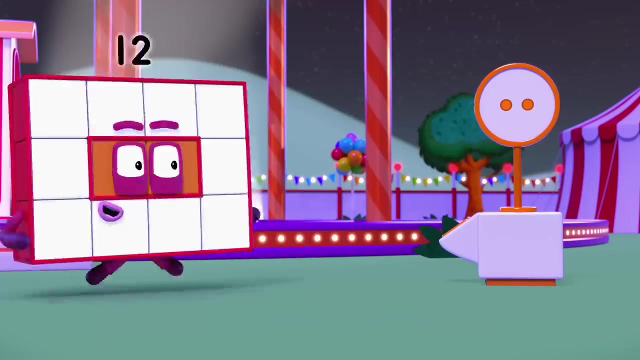 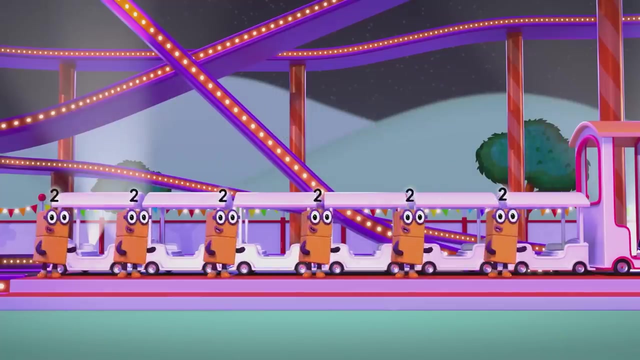 Yay, Now, little ones, are you ready for the fastest, most thrilling most? The Runaway Train. The Runaway Train, Hmm, Haha, In pairs, please Switch All aboard. Two, Two, Two. 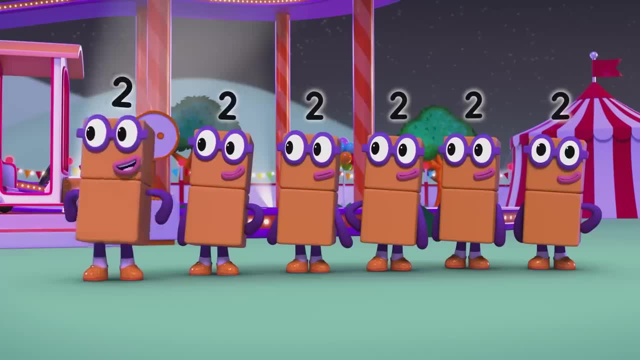 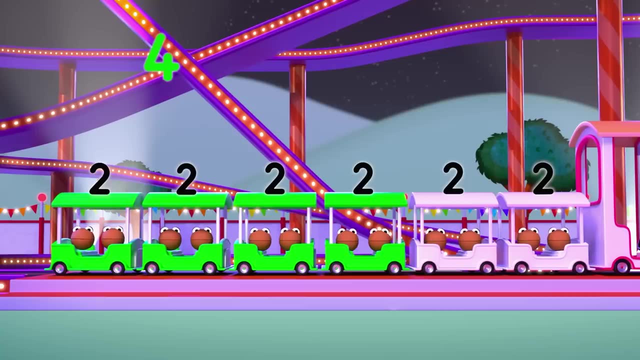 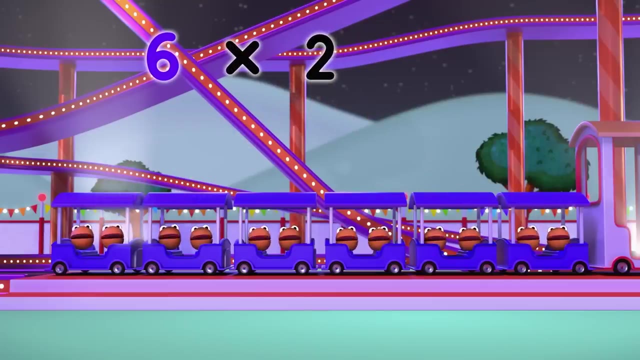 Two, Two, Two. Now how many carriages are there? One, two, three, four, five, six, And how many in each carriage? Two, Six times. So you need 12 more. Oh, I'm all out of tokens. 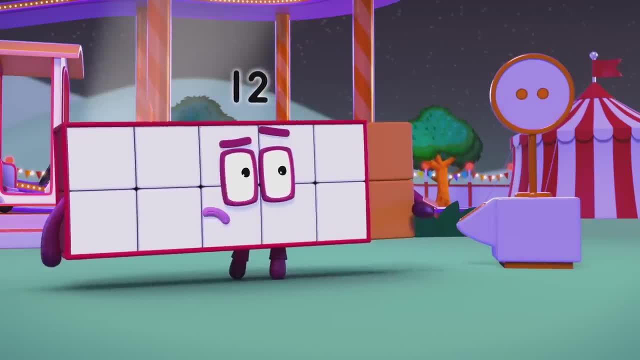 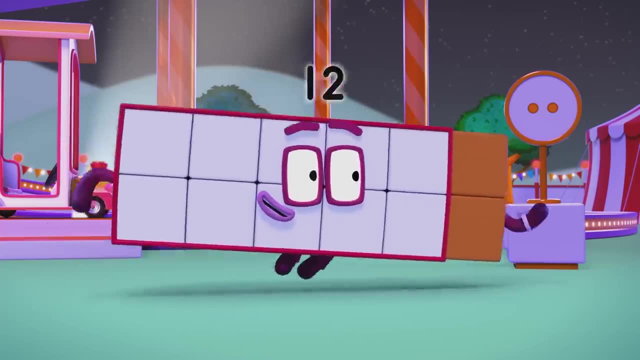 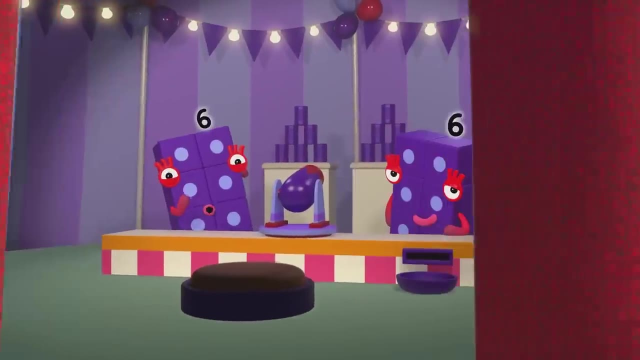 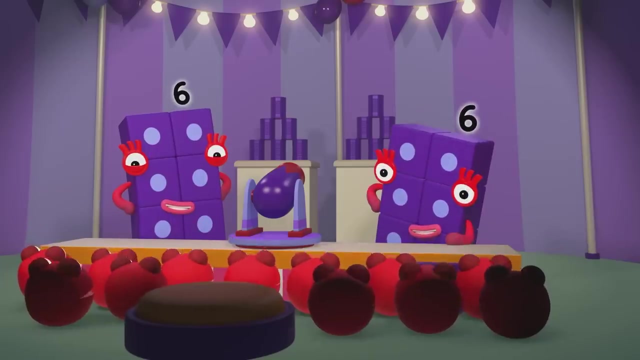 Oh, Ooh, Roll up, roll up and have some fun. There's lots of tokens to be won. Ooh, We need 12 more. Ooh, We need 12 tokens. You'll win one for each can that falls, and there's. 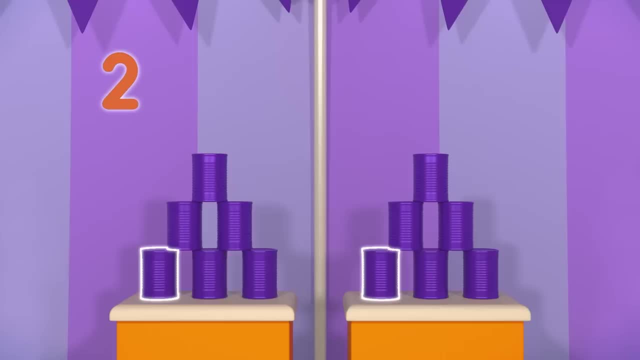 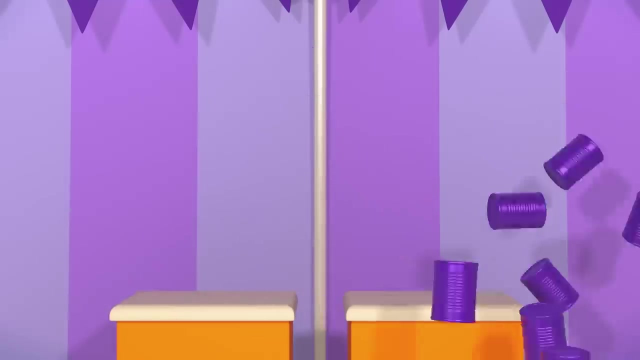 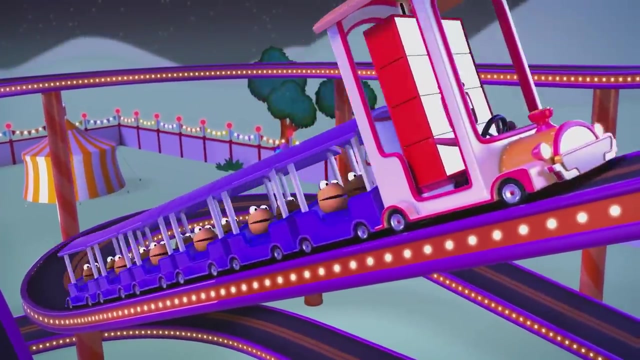 One, two, Two stacks. One, two, three, four, five, six, Six cans in each stack, And two times six equals 12.. Whoa, Hooray, Whoa, Here we go. six, lots of two, twelve numbers of two, two, two, two. 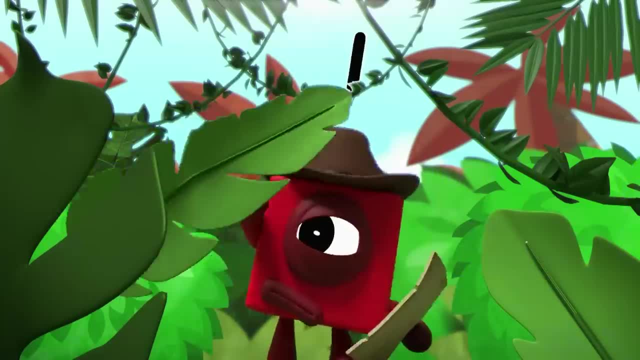 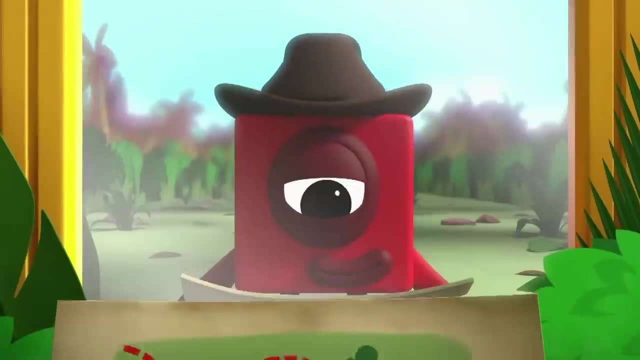 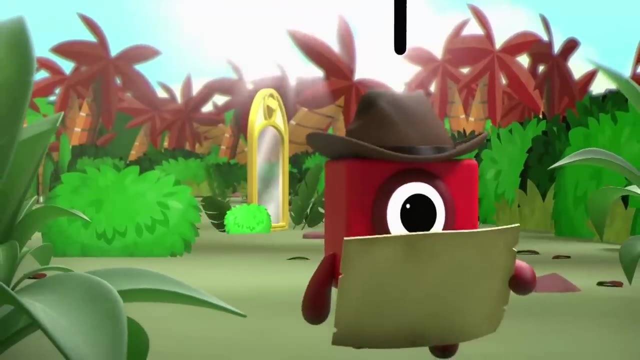 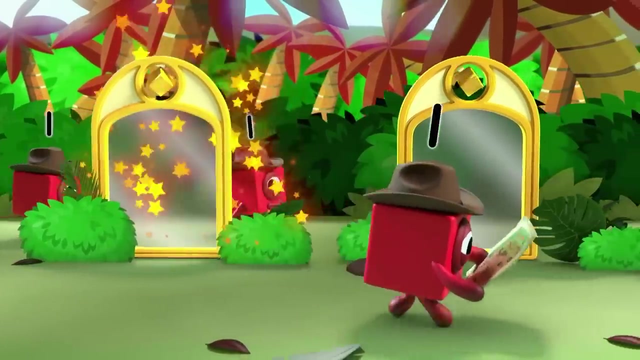 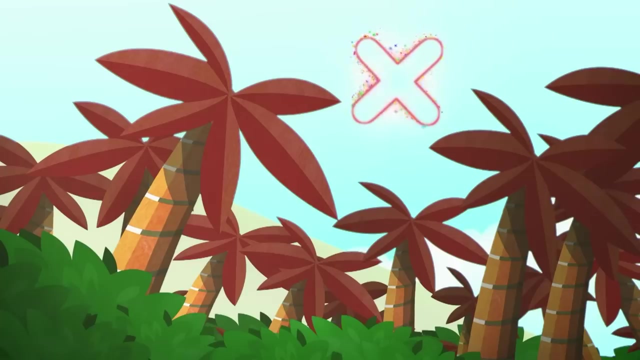 Whoa, Yay, Hmm, X marks the spot. But where is? Ah, Only my reflection. Hello me, That's it. X marks the spot. Hee-hee, Oh, Hee-hee, Oh, Oh. 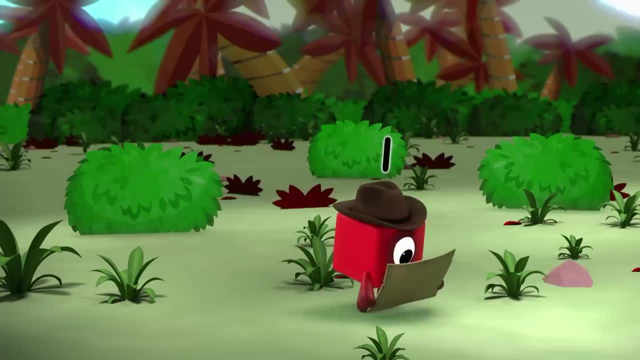 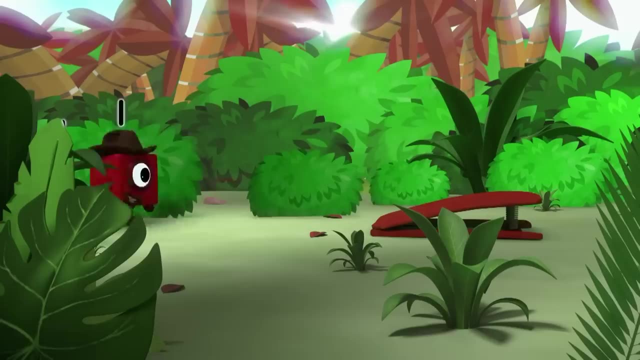 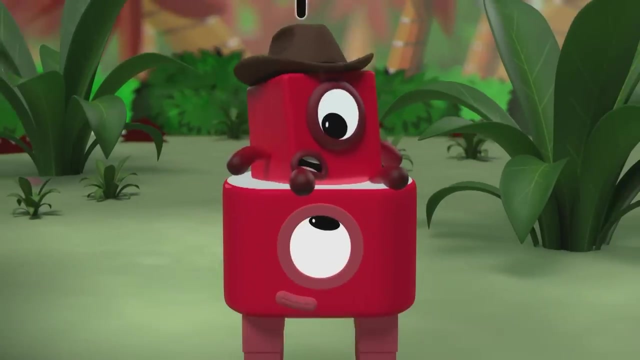 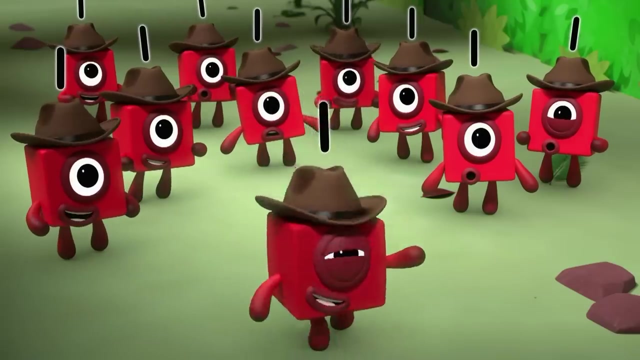 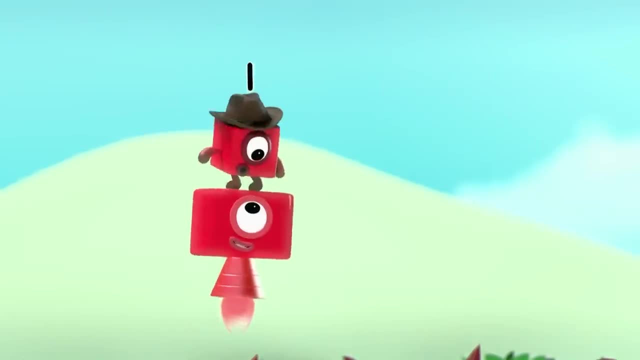 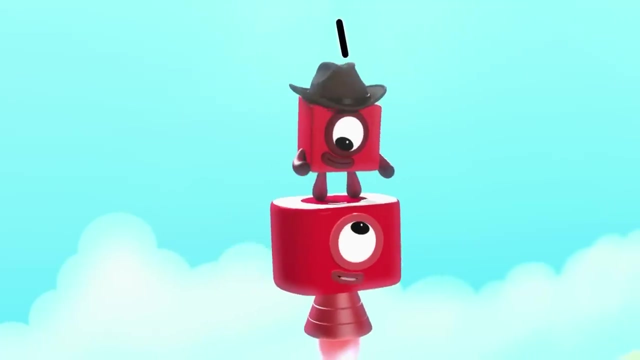 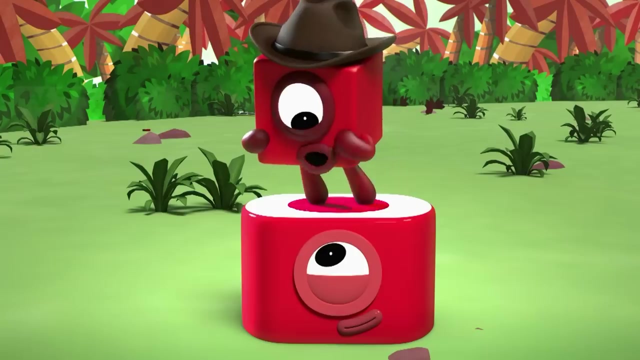 Arrrgh bulbs, Come the lights out, Come with me and you will see I like wands and ones like me. You'll discover What I do never find a label, but you can see i'm one of a kind a table. oh wow, i've never seen a table that. 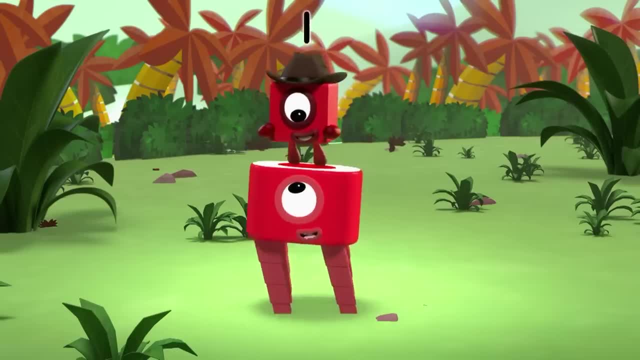 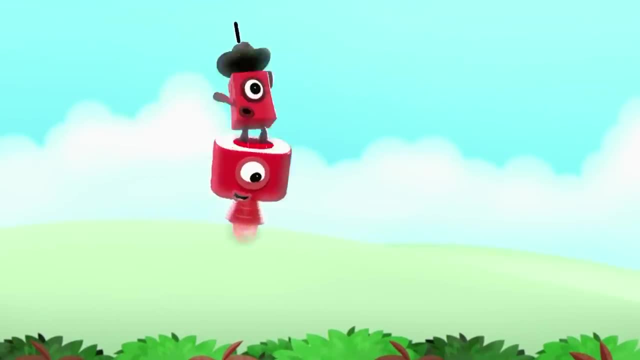 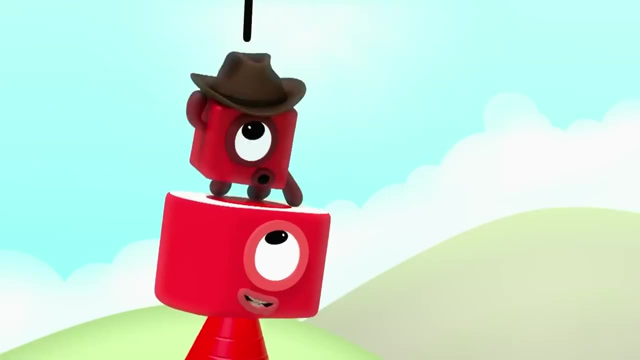 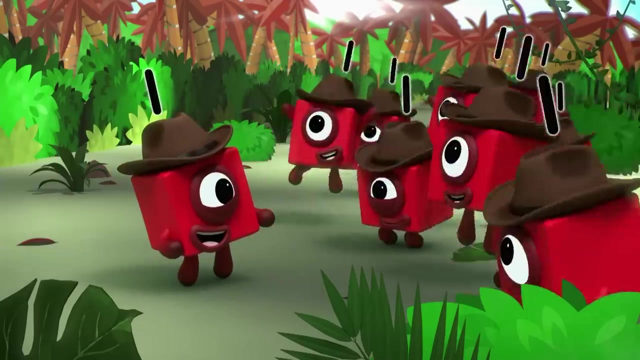 could fly before. well, that's because i'm no ordinary table. i'm the fun times, one times table. in a wonderful world of ones, when it comes to fun, i'm the one who has tons. so sing along, if you're able, for fun times with the one times table, one at a time, please. 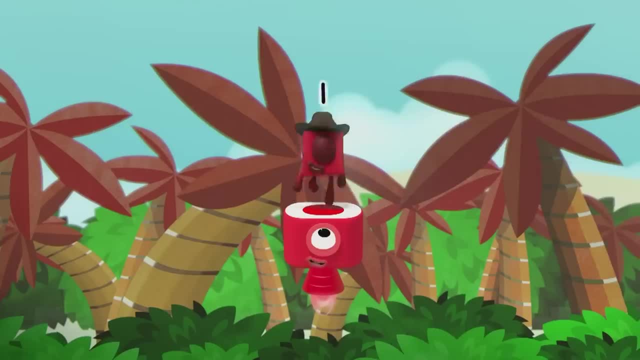 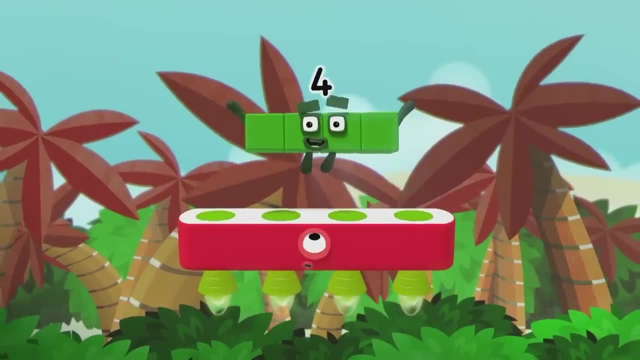 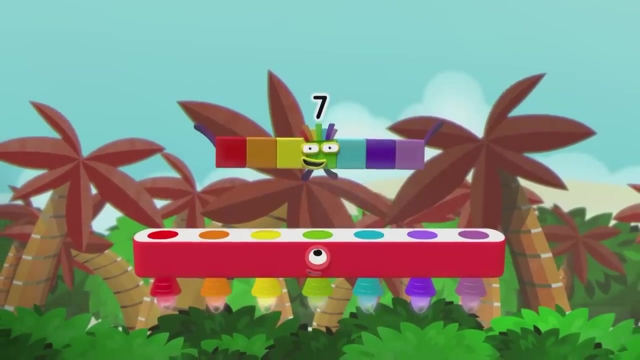 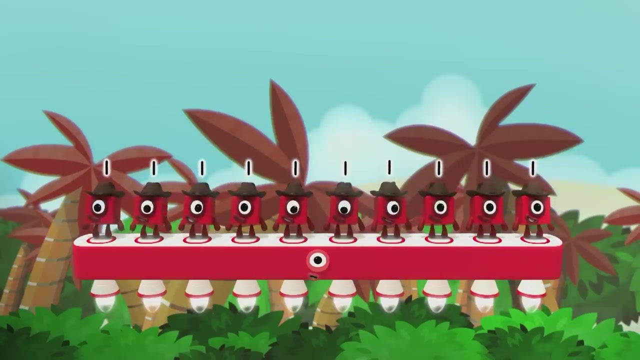 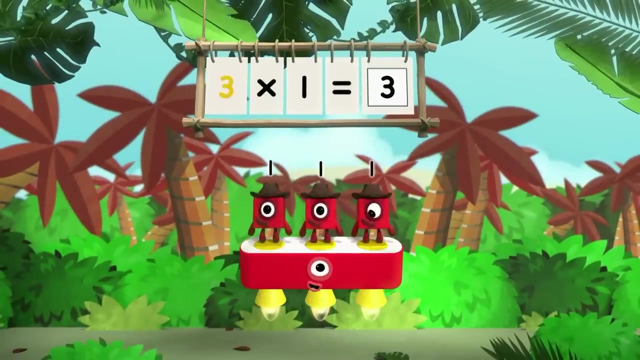 one. one is one, two ones are two, three ones are three, four ones are four, five ones are five, five ones are five, six ones are six and seven ones are seven, eight ones are eight, nine ones are nine and ten ones are ten. sing along: one one is one, two ones are two, three ones are three, four ones are four. 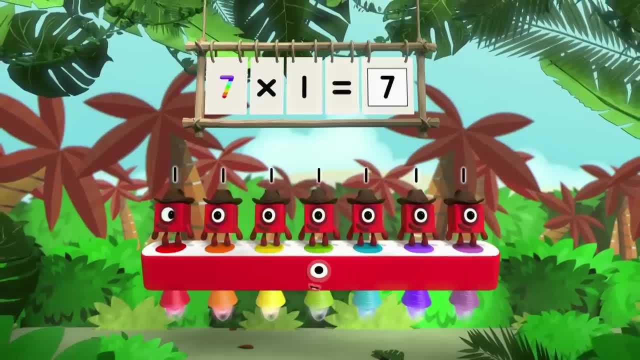 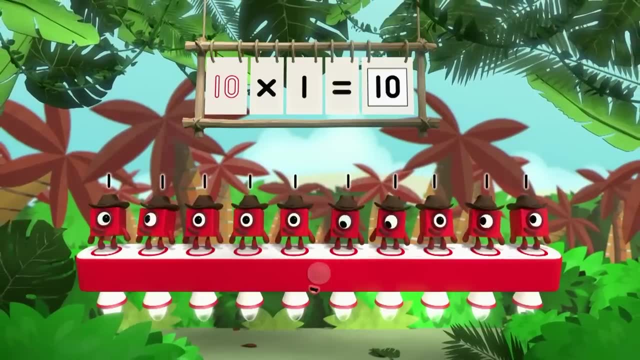 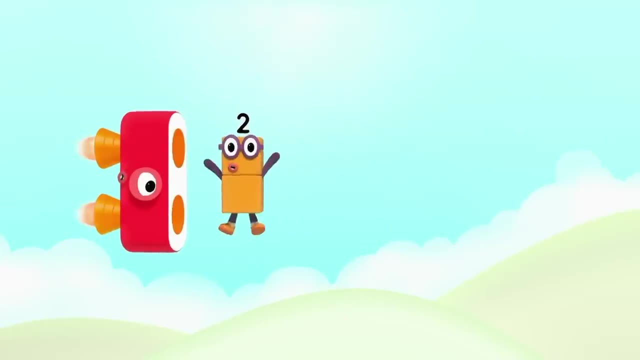 five ones are five, six ones are six and seven ones are seven, eight ones are eight, nine ones are nine and ten ones are ten. sideways, one one is one, two ones are two, three ones are three, four ones are four, five ones are five, six ones are six and seven ones are seven. 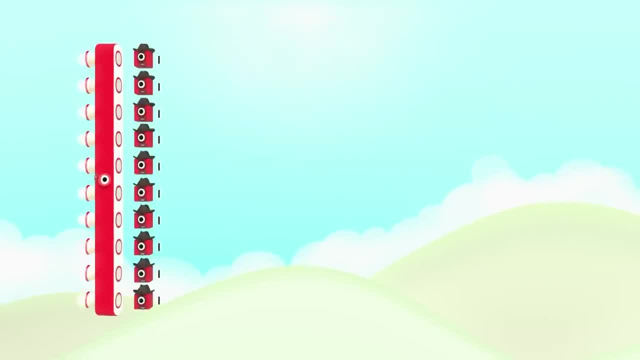 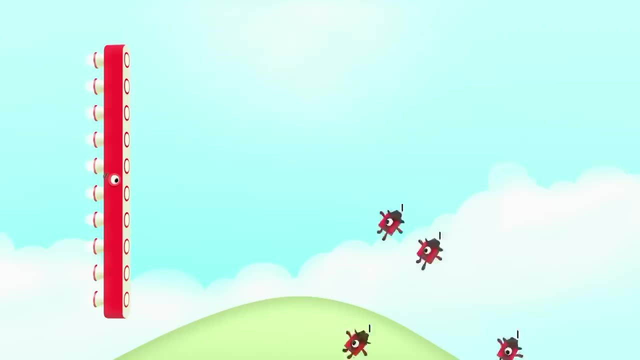 with ones, you can make any number block with ones, you can make any number block now. isn't that clever if you just add now, isn't that clever if you just add now? isn't that clever if you just add one or a bunch of ones, you can go on. 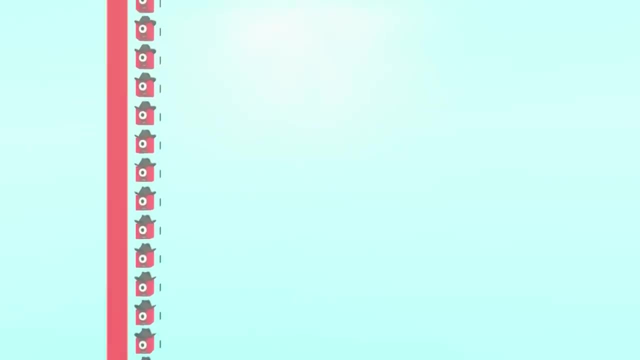 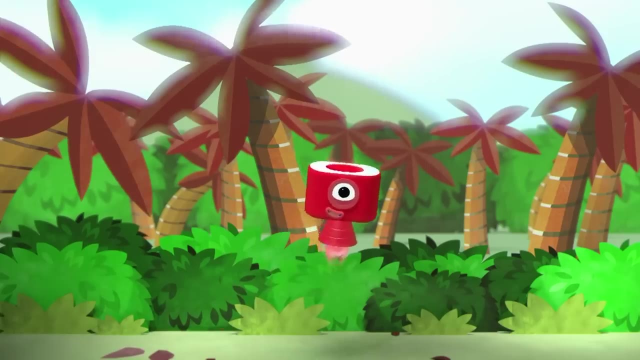 one or a bunch of ones. you can go on one or a bunch of ones. you can go on forever. i'm the fun times, one times table in a. i'm the fun times, one times table in a. i'm the fun times, one times table in a wonderful world of ones. 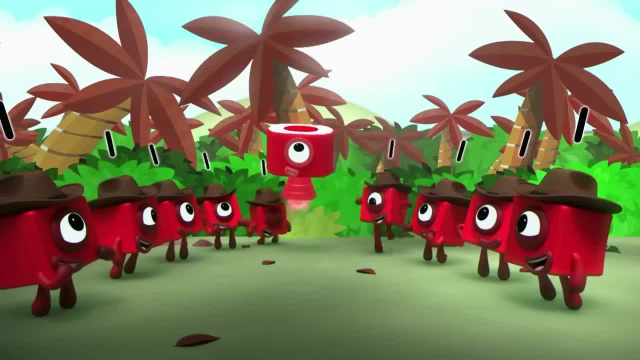 wonderful world of ones. wonderful world of ones. when it comes to fun, i'm the one who has. when it comes to fun, i'm the one who has. when it comes to fun, i'm the one who has tons. so sing along if you're able. tons, so sing along if you're able. 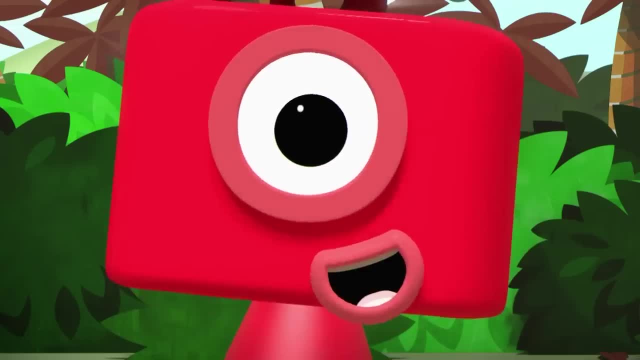 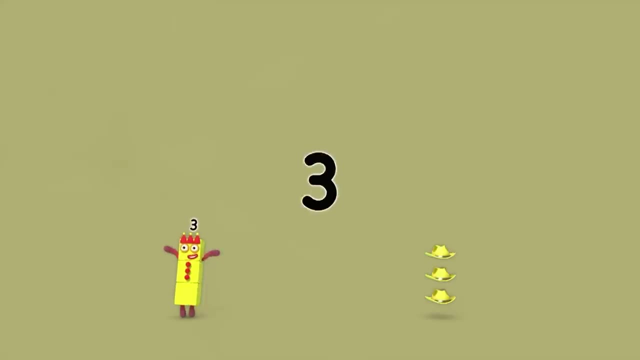 tons. so sing along, if you're able, for fun times with the one times table. for fun times with the one times table. for fun times with the one times table. hats: one hat is one. two hats hats. one hat is one. two hats hats. one hat is one. two hats are two. three hats are three. 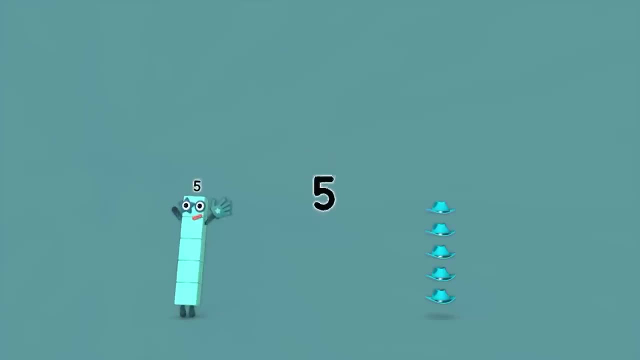 are two. three hats are three are two. three hats are three. four hats are four. five hats are five. four hats are four. five hats are five. four hats are four. five hats are five, six hats are six and seven hats are six. hats are six and seven hats are. 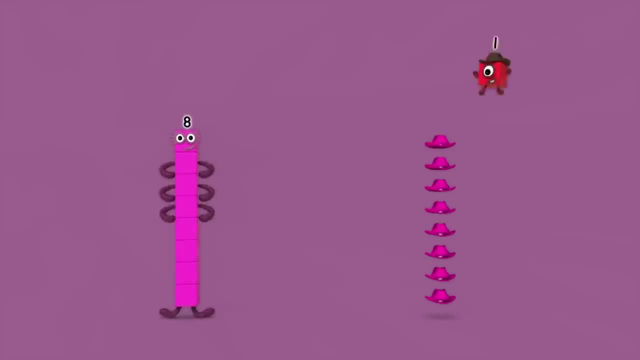 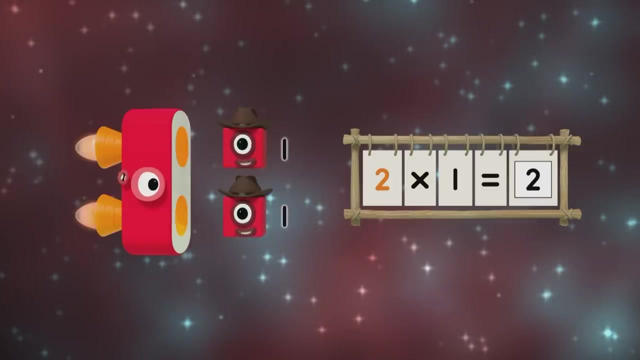 six hats are six and seven hats are seven. seven, seven, eight hats are eight. nine hats are nine. eight hats are eight. nine hats are nine. eight hats are eight. nine hats are nine and ten hats are ten and ten hats are ten and ten hats are ten. one, one is one, two ones are two. 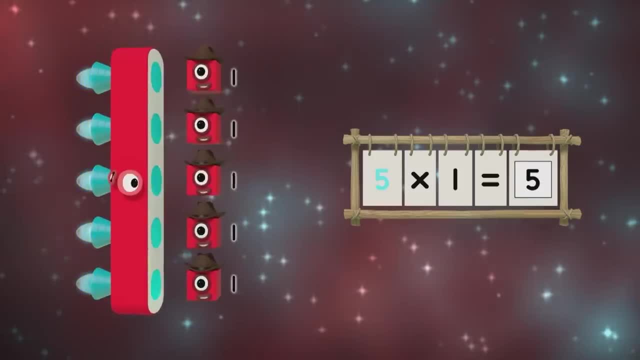 one. one is one, two ones are two. one one is one, two ones are two. three ones are three. four ones are four. three ones are three. four ones are four. three ones are three. four ones are four. five ones are five. six ones are six. five ones are five. six ones are six. 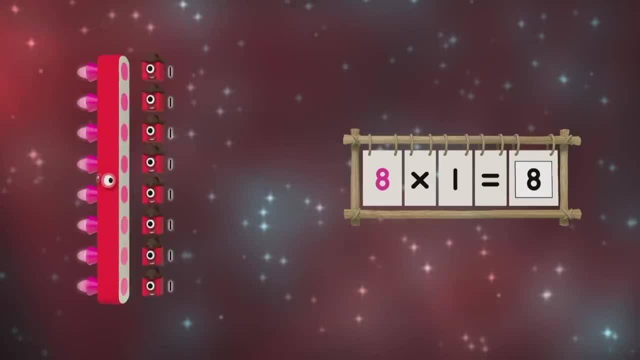 five ones are five, six ones are six and seven ones are seven and seven ones are seven and seven ones are seven, eight ones are eight, nine ones are nine, eight ones are eight, nine ones are nine, eight ones are eight, nine ones are nine, and ten ones and ten ones. 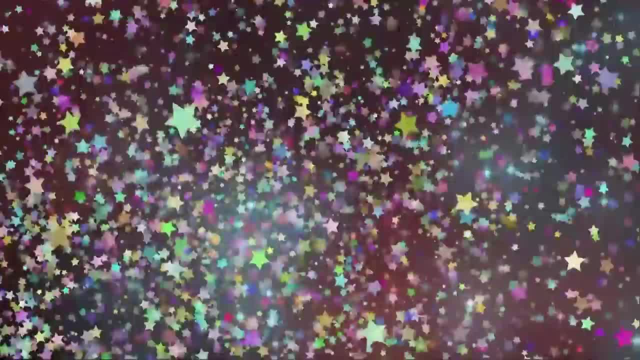 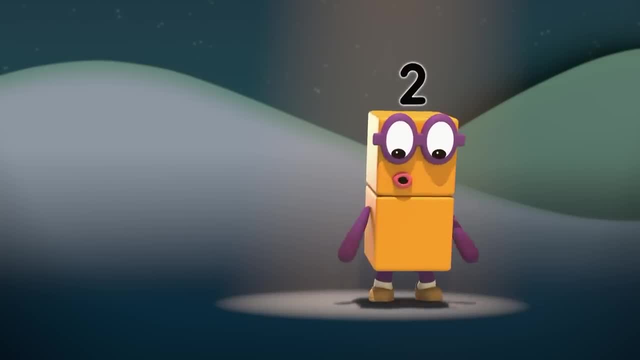 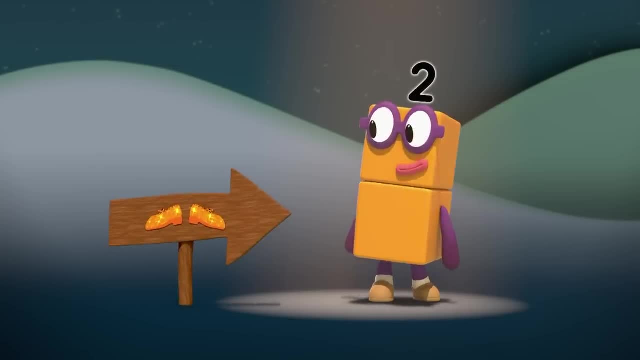 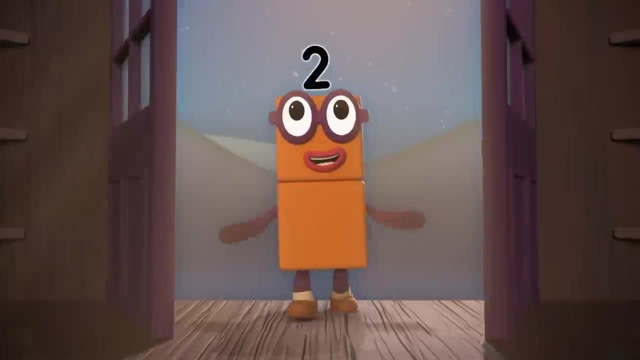 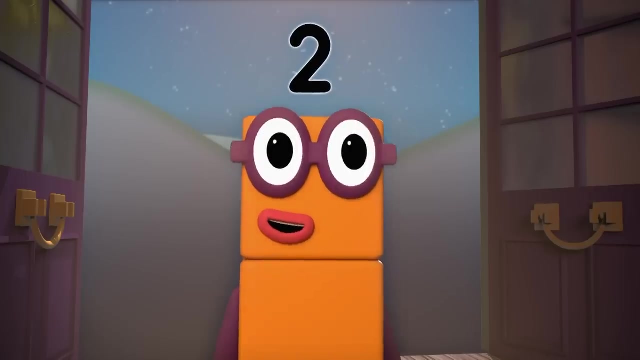 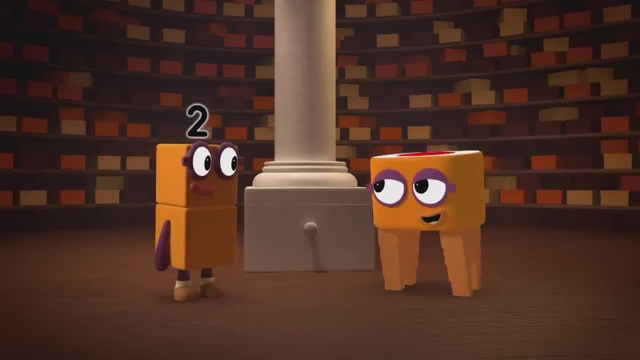 do you like shoes? do you like shoes? well, i like twos. well, i like twos. well, i like twos. i'm the two times table. i'm the two times table, i'm the two times table, and we both like to dance and we both like to dance. 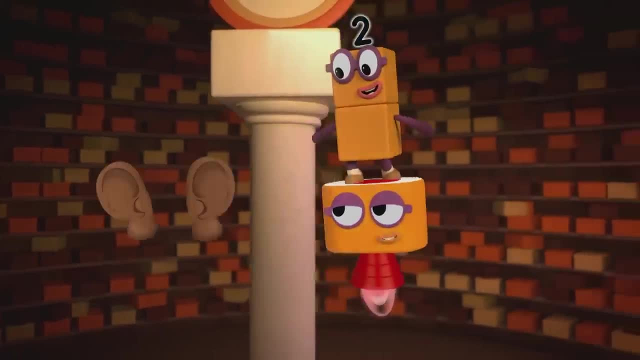 and we both like to dance. i like things that come in twos. i like, i like things that come in twos, i like, i like things that come in twos. i like tears and tears and tears and elbows and knees. i like pairs of gloves, elbows and knees. i like pairs of gloves. 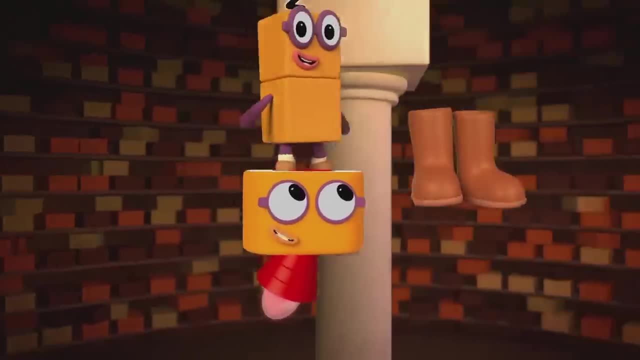 elbows and knees. i like pairs of gloves and turtle doves. i like wings and and turtle doves. i like wings and and turtle doves. i like wings and wellies and water skis. when you're wellies and water skis. when you're wellies and water skis when you're counting slippers or flippers or shoes. 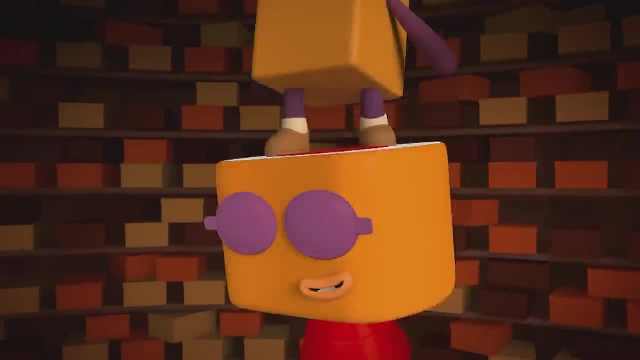 counting slippers or flippers or shoes. counting slippers or flippers or shoes. this is the method you'll need to use a. this is the method you'll need to use a. this is the method you'll need to use a table for twos. table for twos. 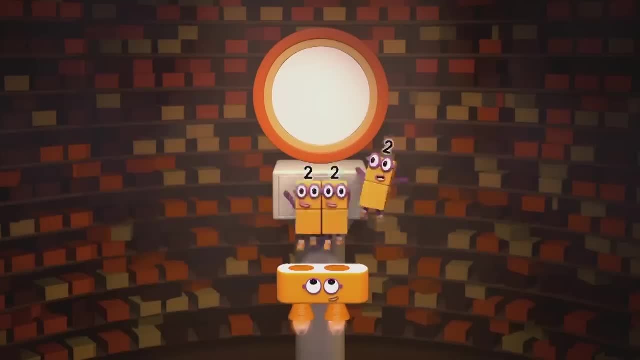 table for twos. one, two is two. two. twos are four. three: one two is two. two. twos are four. three. one two is two. two. twos are four. three. twos are six. are you keeping the score? twos are six. are you keeping the score? 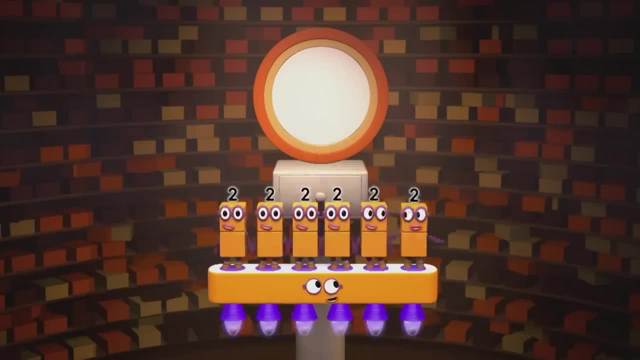 twos are six. are you keeping the score? four twos are eight. five twos are ten. four twos are eight. five twos are ten. four twos are eight. five twos are ten. six twos are 12.. are you ready for more? 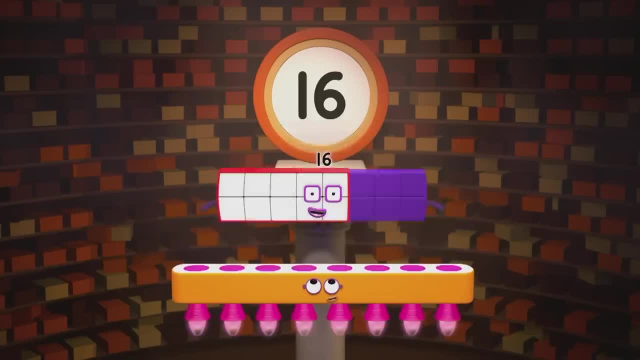 six twos are 12.. are you ready for more? six twos are 12.. are you ready for more? seven twos are 14.. eight seven twos are 14.. eight seven twos are 14.. eight tunes are 16.. nine twos are 18.. that 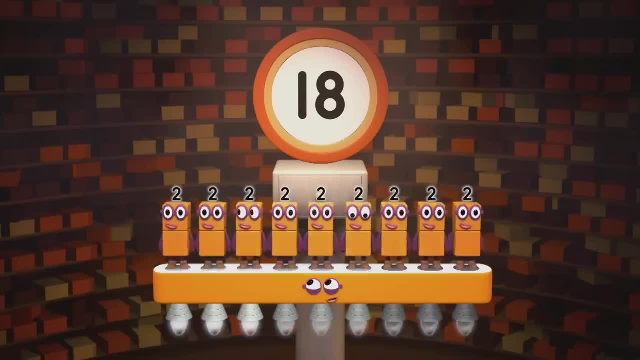 tunes are 16.. nine twos are 18.. that tunes are 16.. nine twos are 18.. that might be plenty, but why should we stop? might be plenty, but why should we stop? might be plenty, but why should we stop now? reach for the top. now: 10 twos. 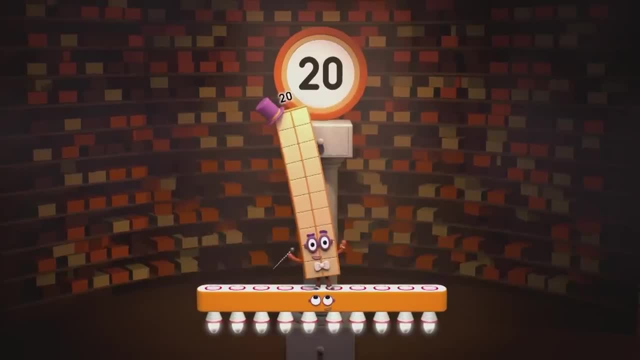 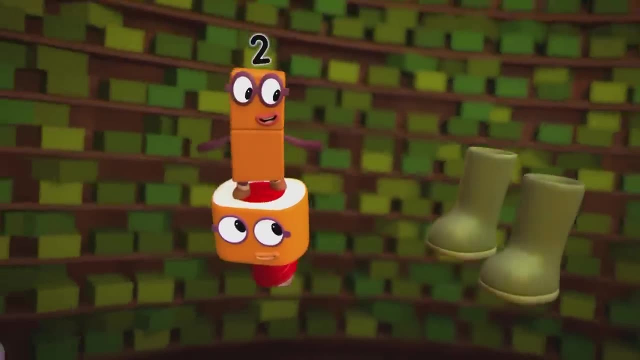 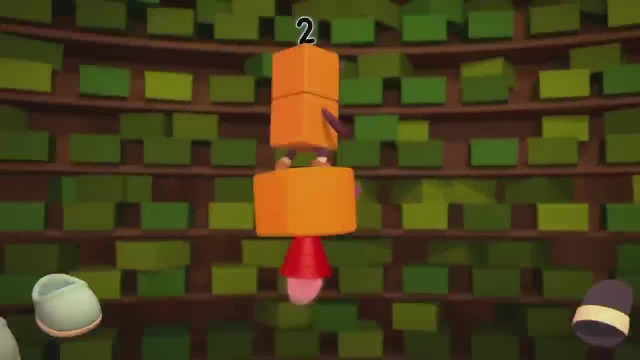 it's shoe time: work. boots and wellies, flip-flops and jellies. slip-ons and flip-flops and jellies. slip-ons and flip-flops and jellies. slip-ons and sliders, sliders, sliders. strength shoes with spikes shiny black. strength shoes with spikes shiny black. 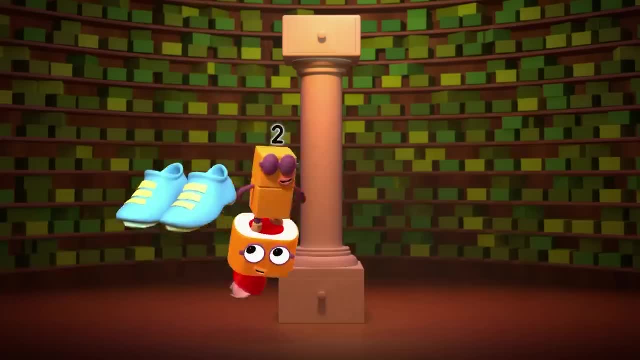 strength shoes with spikes. shiny black tap shoes. tap shoes. tap shoes. buckle and strap shoes. slip bones for buckle and strap shoes. slip bones for buckle and strap shoes. slip bones for riders of super fast bikes- velcro a riders of super fast bikes. velcro- a riders of super fast bikes. velcro- a lace up. let's keep the pace up and 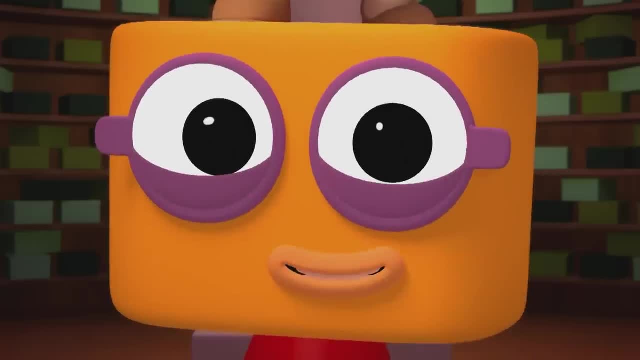 lace up, let's keep the pace up and lace up, let's keep the pace up and count all the shoes, count all the shoes, count all the shoes in twos. one pair is two. two pairs are four, three. one pair is two, two pairs are four, three. 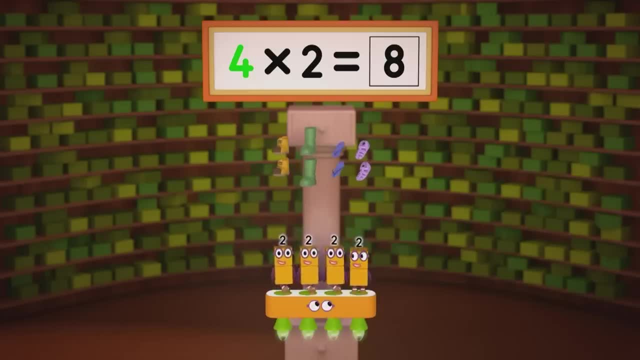 one pair is two. two pairs are four. three pairs are six. now let's take to. the pairs are six. now let's take to. the pairs are six. now let's take to the floor. four pairs are eight. five pairs floor. four pairs are eight. five pairs floor. four pairs are eight. five pairs are ten. six pairs are twelve. you can. 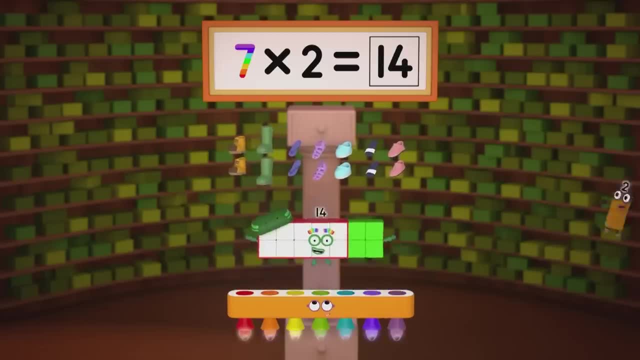 are ten. six pairs are twelve. you can are ten. six pairs are twelve. you can guess what's in store. seven pairs are. guess what's in store. seven pairs are. guess what's in store. seven pairs are fourteen. eight pairs are sixteen. nine. fourteen, eight pairs are sixteen, nine. 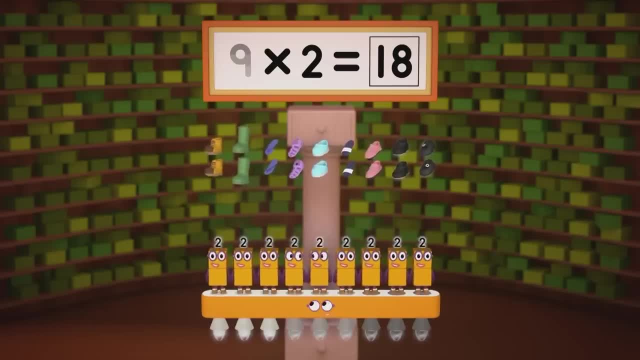 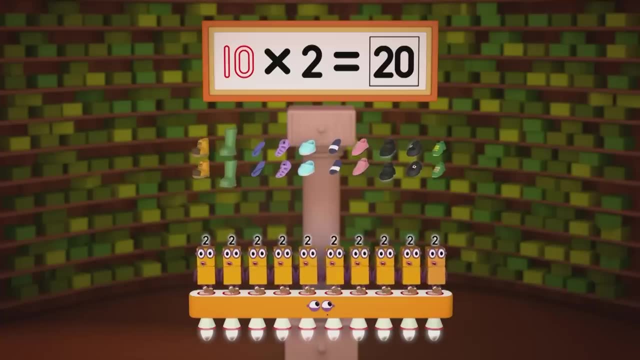 fourteen. eight pairs are sixteen. nine pairs are eighteen. that might be plenty. pairs are eighteen. that might be plenty. pairs are eighteen. that might be plenty, but we can still do more. why not have? but we can still do more. why not have? but we can still do more. why not have two more, ten, two. 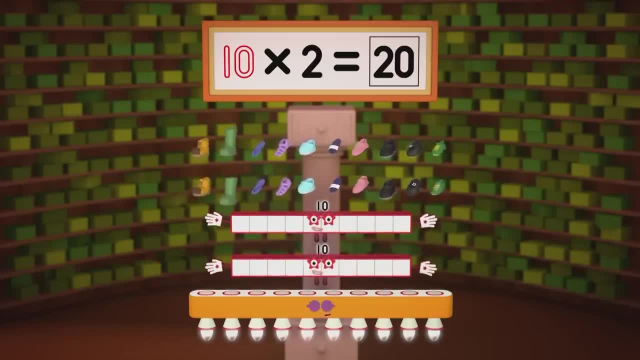 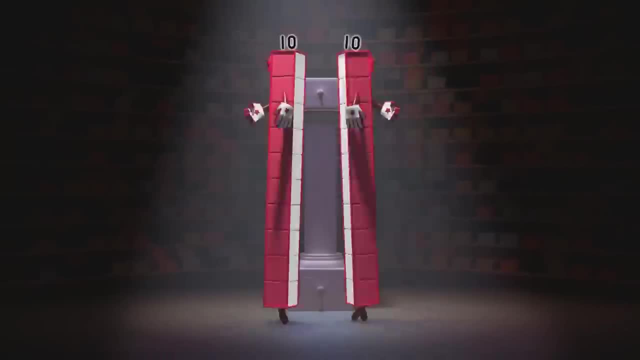 two more ten two. two more ten two are two. tins are two, tins are two, tins are twenty. two tins can tangle and do the fandango. two tins can tangle and do the fandango. two tins can tangle and do the fandango. twenty unstoppable swappable blocks. 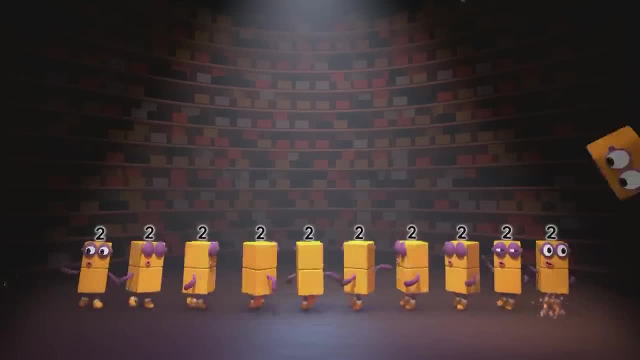 twenty unstoppable swappable blocks. twenty unstoppable swappable blocks. ten twos can line up and shine up their ten twos can line up and shine up. their ten twos can line up and shine up their shoes, shoes, shoes- where there are shoes, there are usually. where there are shoes, there are usually. 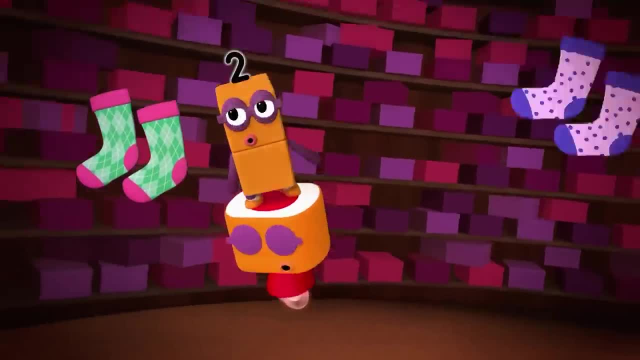 where there are shoes, there are usually socks, socks, socks strappy and spotty diamond and dotty strappy and spotty diamond and dotty strappy and spotty diamond. and dotty yellow and red. socks with yellow and red. socks with yellow and red. socks with holes in the toes. long socks and short. 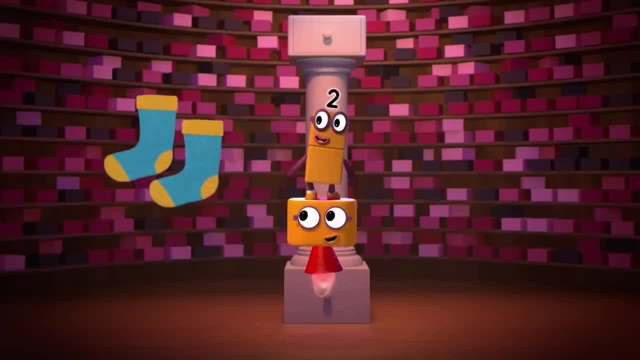 holes in the toes. long socks and short. holes in the toes. long socks and short socks. school socks and sports socks. warm socks, school socks and sports socks. warm socks, school socks and sports socks. warm woolly bed socks, which grandma once. woolly bed socks, which grandma once. 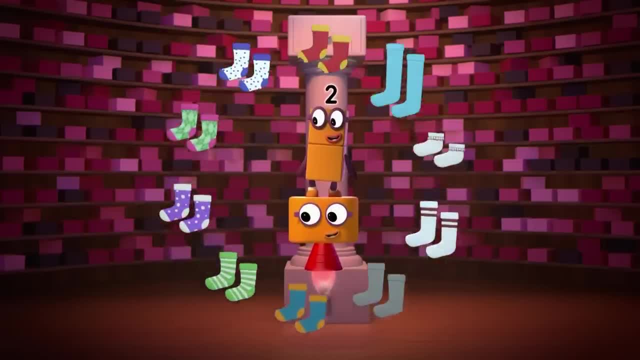 woolly bed socks, which grandma once chose. silky and snazzy. jolly and jazzy chose silky and snazzy. jolly and jazzy chose silky and snazzy. jolly and jazzy. let's count them all. let's count them all. 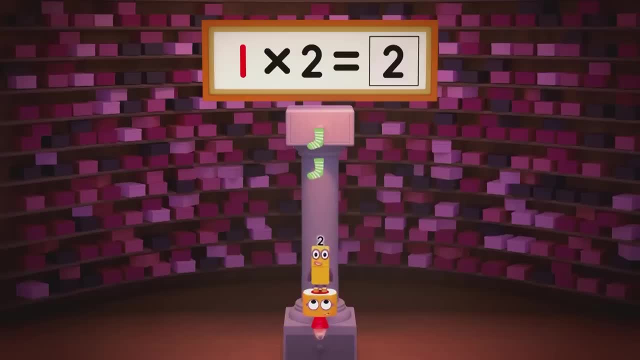 let's count them all. good call, good call, good call. one pair is two. two pairs are four. one pair is two. two pairs are four. one pair is two. two pairs are four. three pairs are six. now let's open the. three pairs are six. now let's open the. 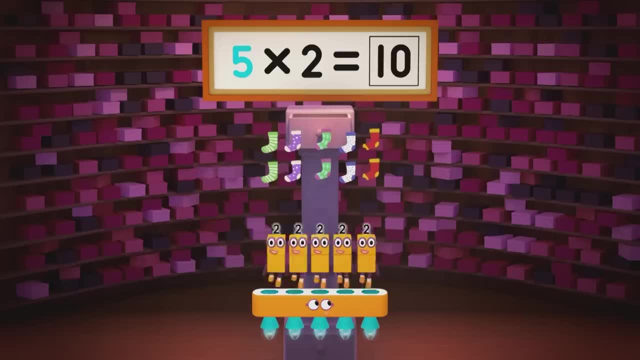 three pairs are six. now let's open the drawer. four pairs are eight. five pairs drawer. four pairs are eight. five pairs drawer. four pairs are eight. five pairs are ten. six pairs are twelve socks. you are ten. six pairs are twelve socks. you are ten. six pairs are twelve socks. you cannot ignore seven pairs of fourteen. 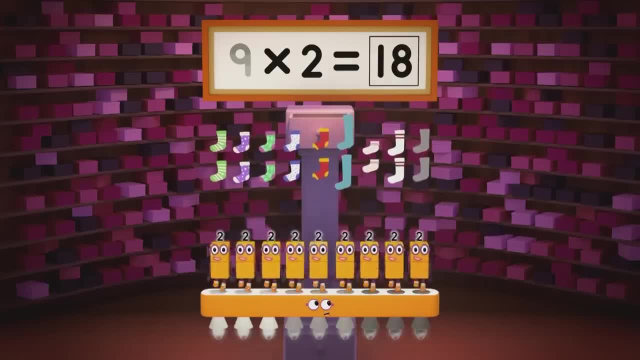 cannot ignore seven pairs of fourteen. cannot ignore seven pairs of fourteen. eight pairs are sixteen. nine pairs are eight. pairs are sixteen. nine pairs are eight. pairs are sixteen. nine pairs are eighteen. that might be plenty. eighteen, that might be plenty. eighteen, that might be plenty. let's have some new socks, orange and 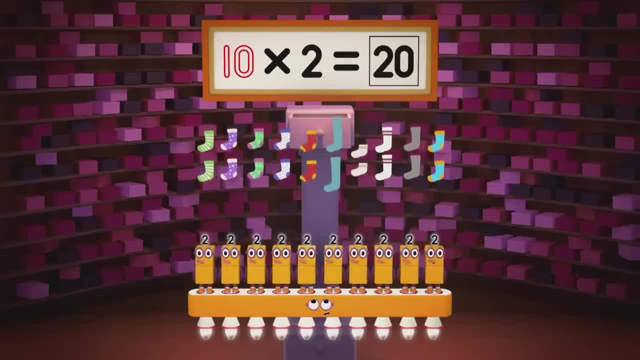 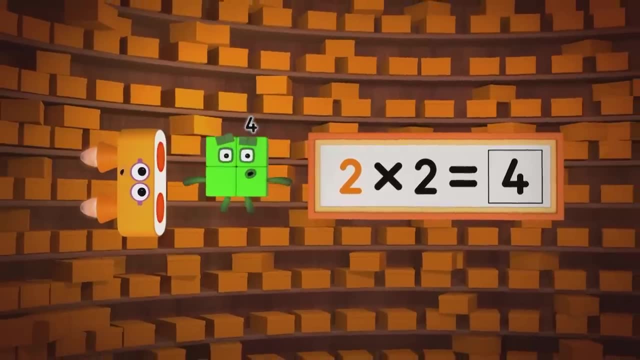 let's have some new socks orange, and let's have some new socks orange and blue socks. ten pairs blue socks, ten pairs blue socks. ten pairs are twenty, are twenty, are twenty sideways, sideways, sideways. one, two is two, one, two is two, one, two is two. two, one, two is two, two, twos are four, three, twos are six. 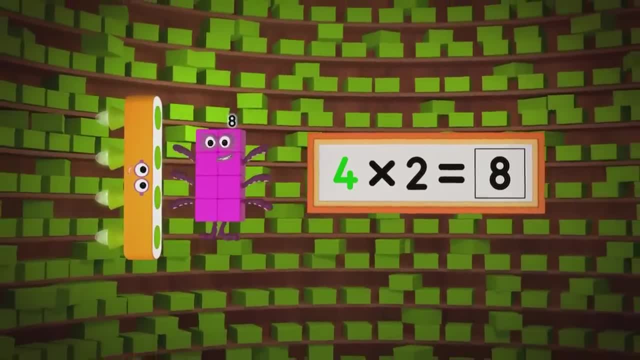 twos are four. three twos are six. twos are four. three twos are six. are you keeping the score? four twos are. are you keeping the score? four twos are. are you keeping the score? four twos are eight. five twos are ten. six twos are. 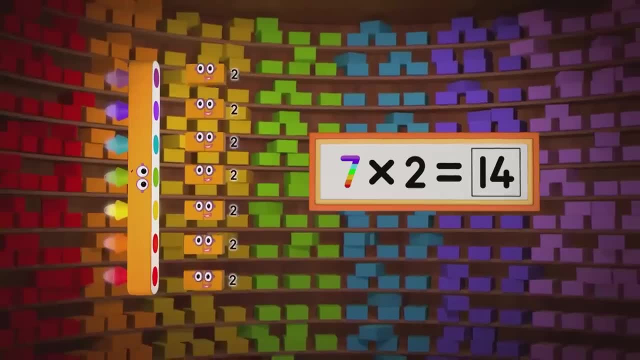 eight. five twos are ten. six twos are eight. five twos are ten. six twos are twelve. are you ready for more twelve? are you ready for more twelve? are you ready for more? seven twos are fourteen. eight twos are seven. twos are fourteen. eight twos are: 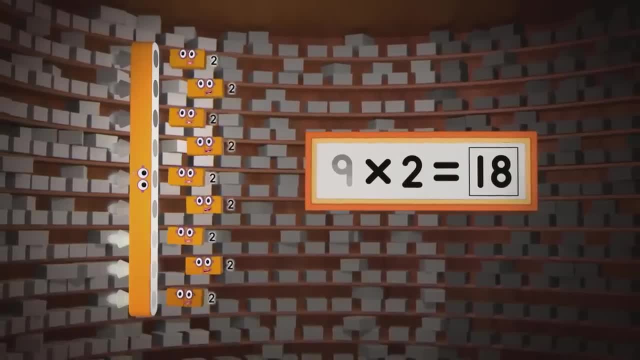 seven twos are fourteen, eight twos are sixteen, nine twos are eighteen. that sixteen nine twos are eighteen, that sixteen nine twos are eighteen. that might be plenty, might be plenty, might be plenty, but why should we stop now reach for the? but why should we stop now reach for the? 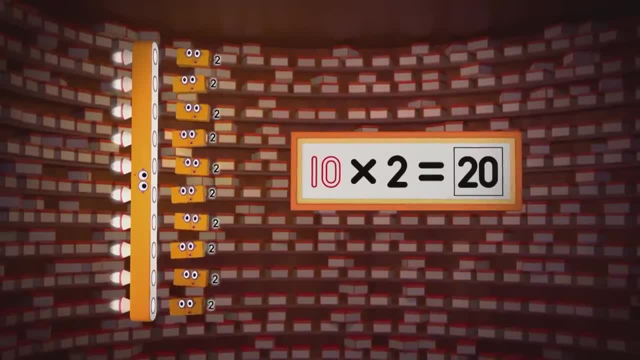 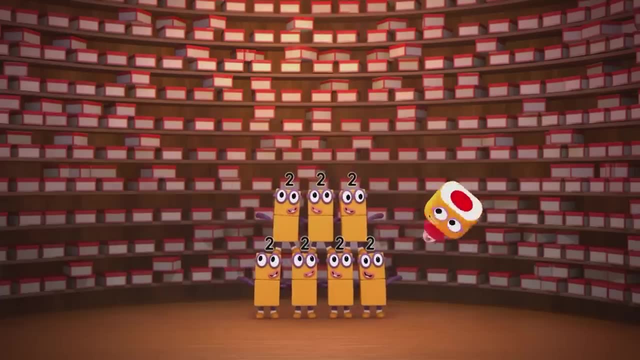 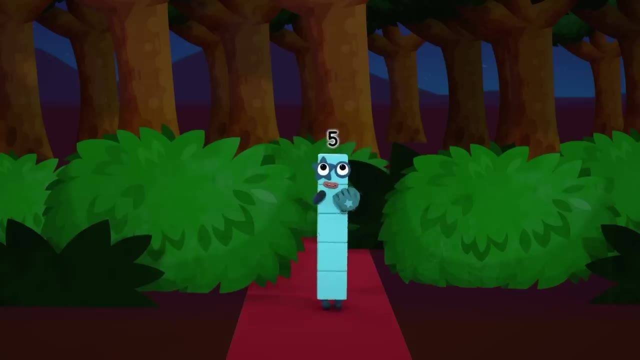 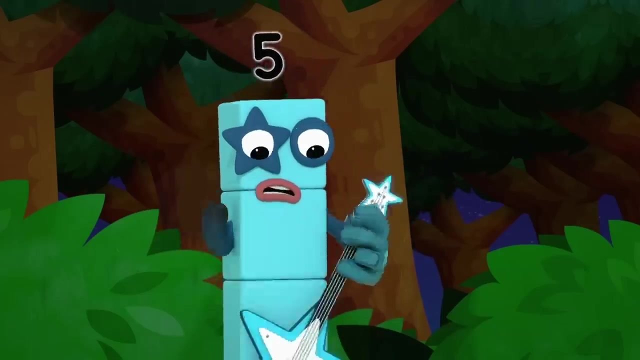 but why should we stop now? reach for the top now. ten twos: wow, that's here. that's a real wow. that's here, that's a real wow. that's here, that's a real. the tower of rock. but am i good enough? yes, of course you. 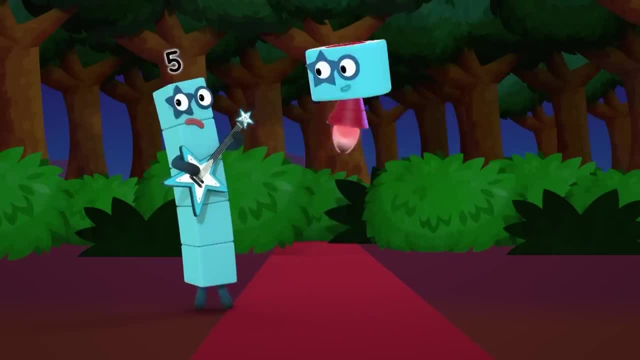 but am i good enough? yes, of course you. but am i good enough? yes, of course you are, are, are huh, huh, huh, huh. you've got talent, you've got drive. and you've got talent, you've got drive and you've got talent, you've got drive, and you never give up. 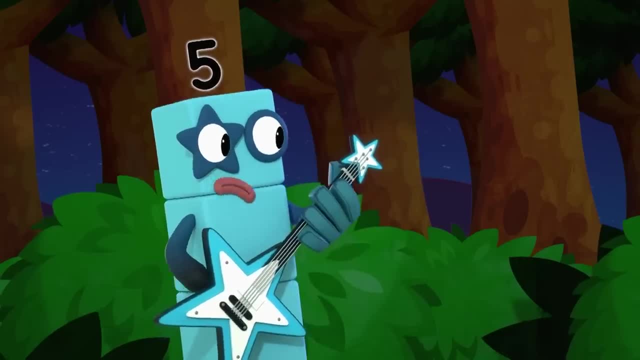 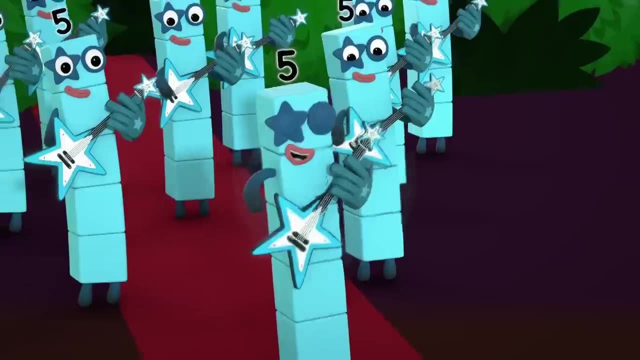 you never give up. you never give up. it runs in the family, the family, the family of fives high five, the family of fives high five, the family of fives high five. let's rock, let's rock, let's rock, crack it up, crack it up. 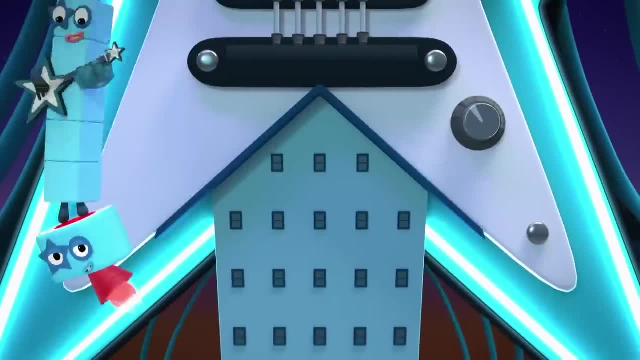 crack it up. plug in the cable, plug in the cable, plug in the cable. i'm the one and only five-time sable. i'm the one and only five-time sable. i'm the one and only five-time sable. it's time to come alive and meet your. 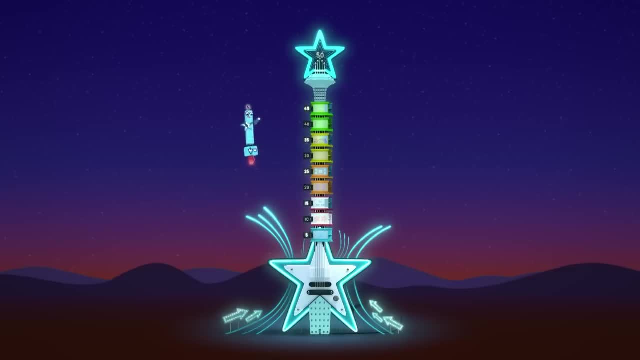 it's time to come alive and meet your. it's time to come alive and meet your heroes, heroes, heroes. some of them end in five and some end. some of them end in five and some end. some of them end in five and some end in zero, in zero. 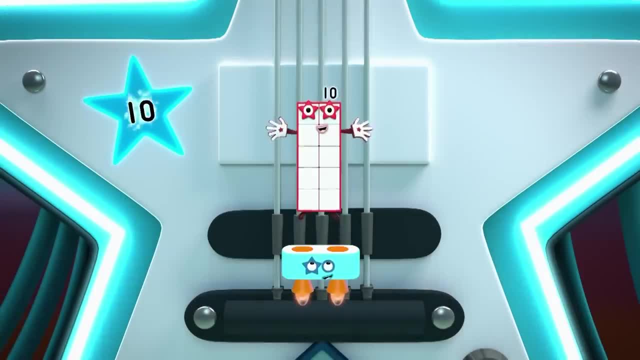 in zero. one five is five. two fives are ten. one five is five. two fives are ten. one five is five. two fives are ten. three fives are fifteen. trust me, you'll go. three fives are fifteen. trust me, you'll go. three fives are fifteen. trust me, you'll go far. 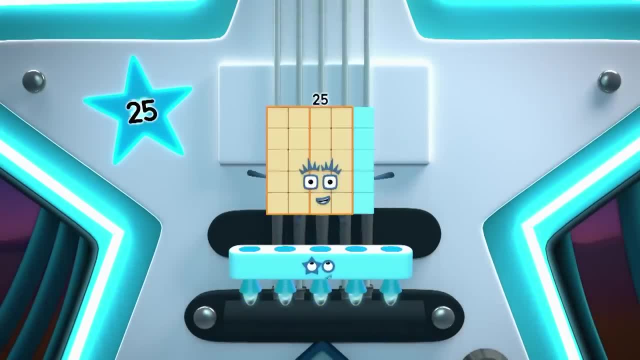 far, far. four fives are twenty five. fives are four, fives are twenty five. fives are four, fives are twenty five. fives are twenty five. six fives are thirty. you know twenty five, six fives are thirty. you know, twenty five, six fives are thirty. you know who you are. 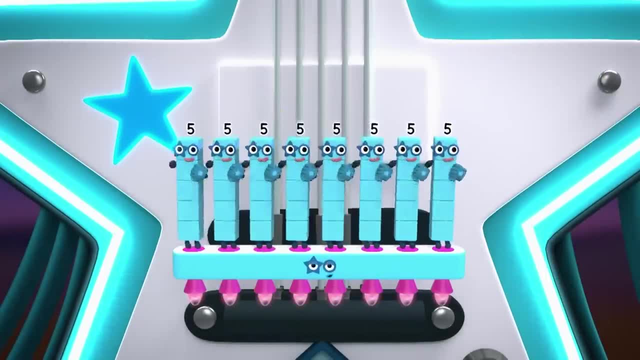 who you are, who you are. seven fives are thirty-five. eight fives, seven fives are thirty-five. eight fives, seven fives are thirty-five. eight fives are forty nine fives are forty five and are forty nine fives are forty five and. 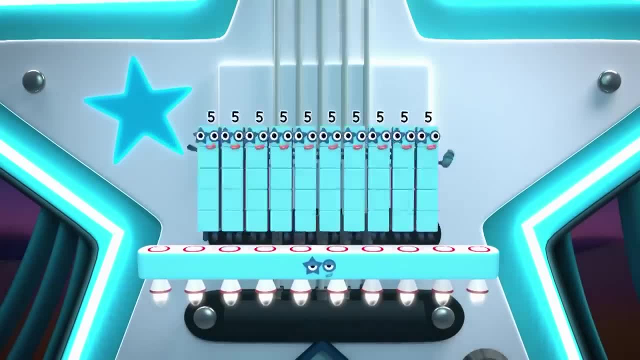 are forty. nine fives are forty five. and here's the next big superstar. ten fives, here's the next big superstar. ten fives. here's the next big superstar. ten fives are fifty. take it to the top. are fifty. take it to the top. are fifty. take it to the top. one five will land her hand. she's the. 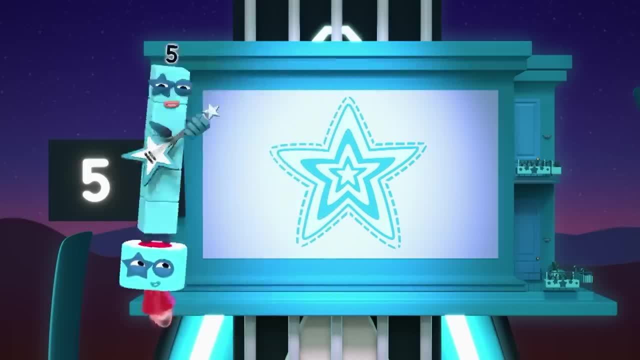 one five will land her hand. she's the one five will land her hand. she's the leader of the band five. leader of the band five. leader of the band five, high five. two fives can take a trip. they can make. two fives can take a trip, they can make. 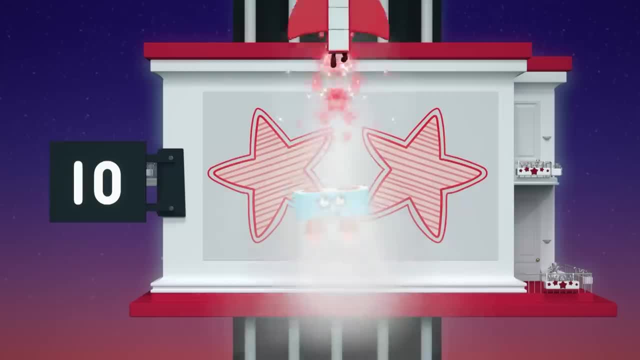 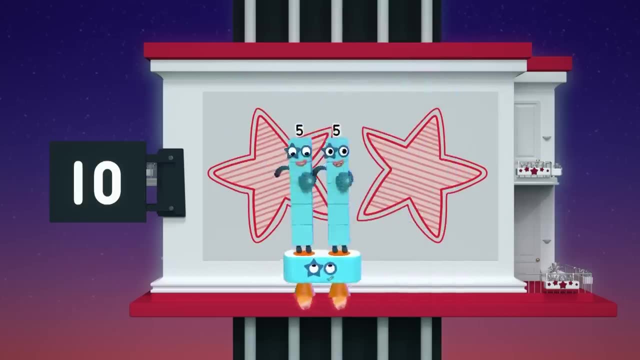 two, fives can take a trip. they can make a rocket ship, a rocket ship, a rocket ship. lost, all lost, all lost, all. cause i'm the five times table, cause i'm the five times table, cause i'm the five times table, stop me up and we'll go up in five. 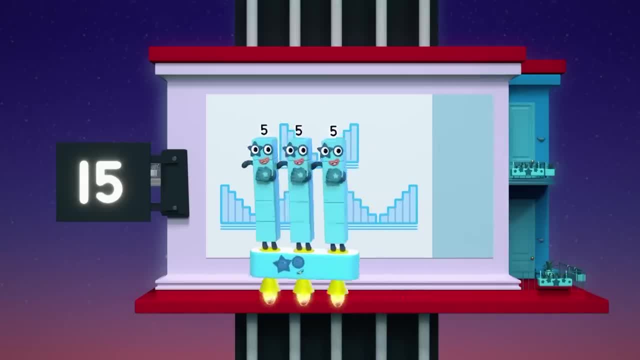 stop me up and we'll go up in five. stop me up and we'll go up in five. three fives are slightly odd. they're a. three fives are slightly odd. they're a. three fives are slightly odd. they're a secret special squad 15.. 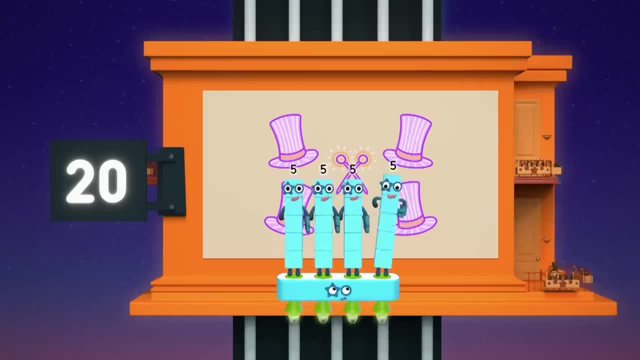 secret special squad 15.. secret special squad 15. hush, hush, slightly odd. hush, hush, slightly odd. hush, hush, slightly odd. four fives make a great quartet, but you four fives make a great quartet. but you four fives make a great quartet, but you ain't seen nothing yet. 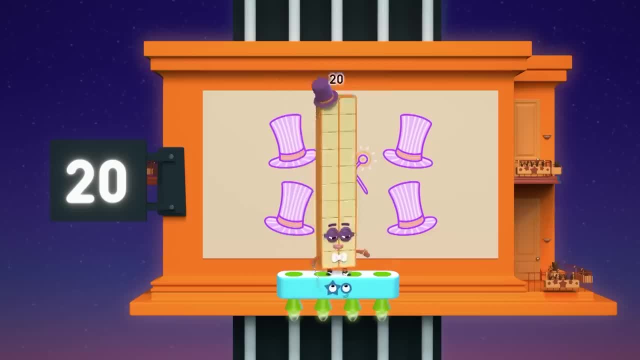 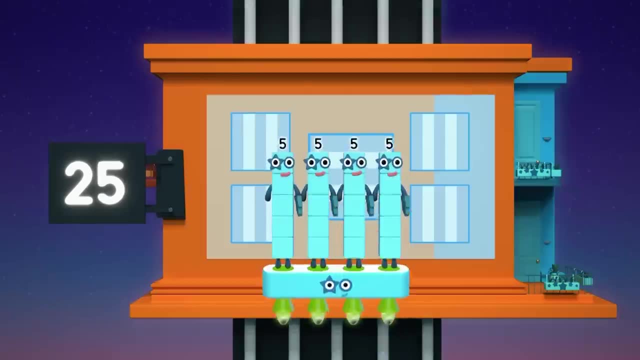 ain't seen nothing yet. ain't seen nothing yet. twenty, twenty, twenty, cause i'm the five times table. stop me up, cause i'm the five times table. stop me up, cause i'm the five times table. stop me up and we'll go up in five, and we'll go up in five. 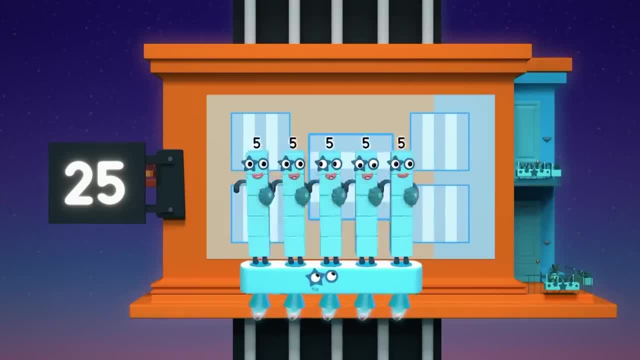 and we'll go up in five. five fives were halfway there. five, fives, five, fives were halfway there. five, fives, five, fives were halfway there. five, fives make a great big square. twenty-five make a great big square. twenty-five make a great big square. twenty-five square. six, fives are neatly stacked six. 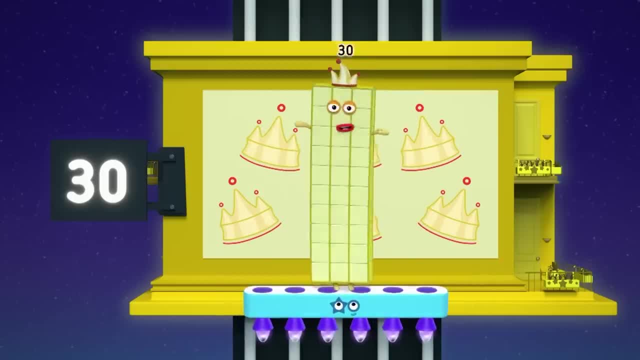 square. six fives are neatly stacked. six square. six fives are neatly stacked. six fives are a circus act. fives are a circus act. fives are a circus act. the greatest show in number land, the greatest show in number land, the greatest show in number land: seven fives never come unstuck. seven. 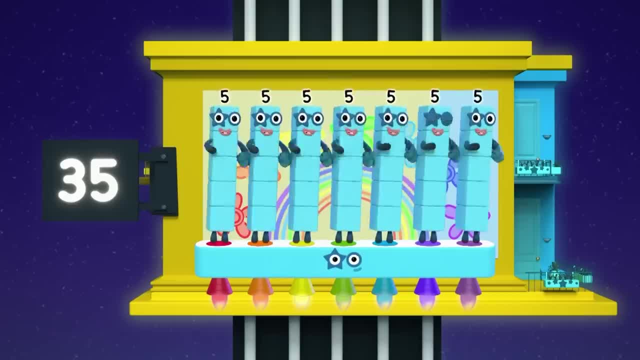 seven fives never come unstuck. seven, seven fives never come unstuck. seven fives have sevens. look, thirty-five fives have sevens. look, thirty-five fives, have sevens. look, thirty-five, eight fives, we're getting bigger they, eight fives, we're getting bigger they. 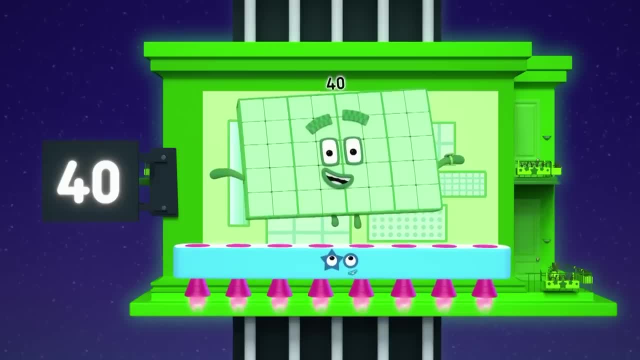 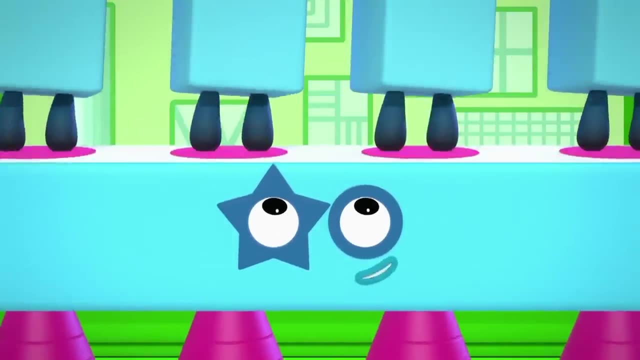 eight, fives. we're getting bigger. they make an impressive figure. make an impressive figure, make an impressive figure. forty, forty, forty, cause i'm a five times table. stop me up, cause i'm a five times table. stop me up cause i'm a five times table. stop me up and we'll go up in five. 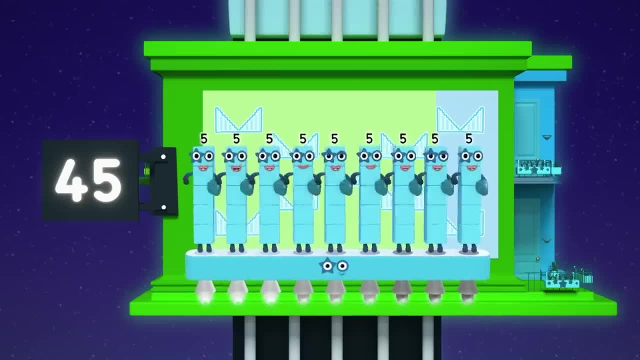 and we'll go up in five, and we'll go up in five. nine fives. step up the pace and take you nine fives. step up the pace and take you nine fives. step up the pace and take you to a higher place, to a higher place. 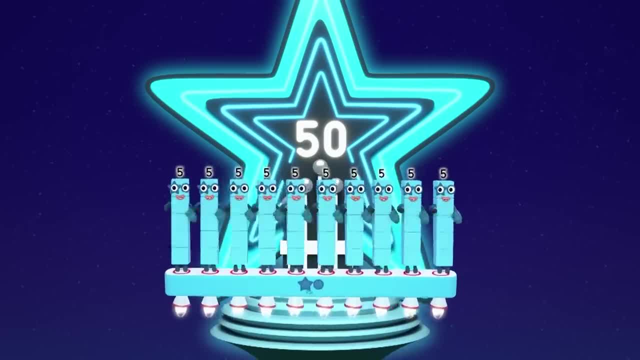 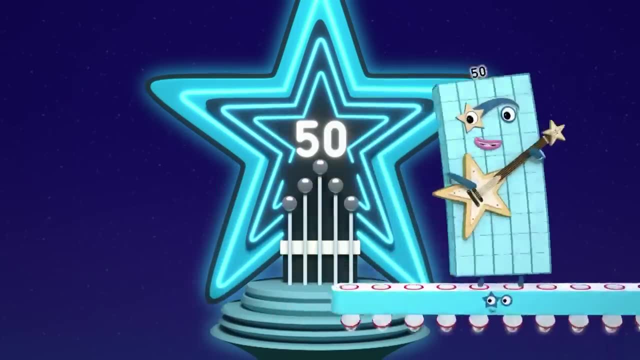 to a higher place. forty-five, ten fives with a gold guitar. forty-five, ten fives with a gold guitar. forty-five, ten fives with a gold guitar. ten fives make a superstar. ten fives make a superstar. ten fives make a superstar high. fifty: 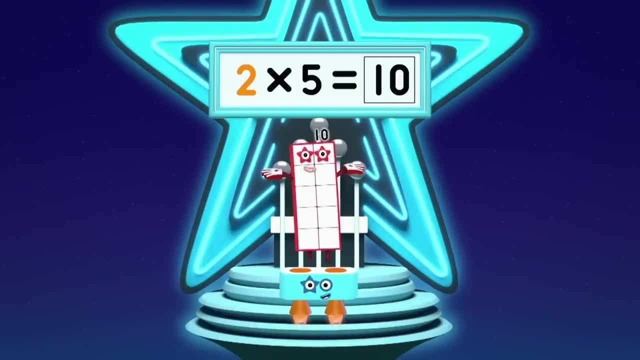 high fifty, high fifty. one five is five. two fives are ten. one five is five. two fives are ten. one five is five. two fives are ten. three fives are fifteen. trust me you'll. three fives are fifteen. trust me you'll. three fives are fifteen. trust me, you'll go far. 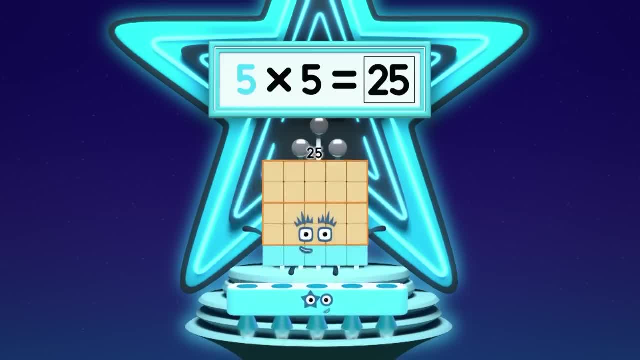 go far, go far. four fives are twenty five. fives are four. fives are twenty five. fives are four. fives are twenty five. fives are twenty five. six fives are thirty. twenty five, six fives are thirty. twenty five, six fives are thirty. you know who we are. 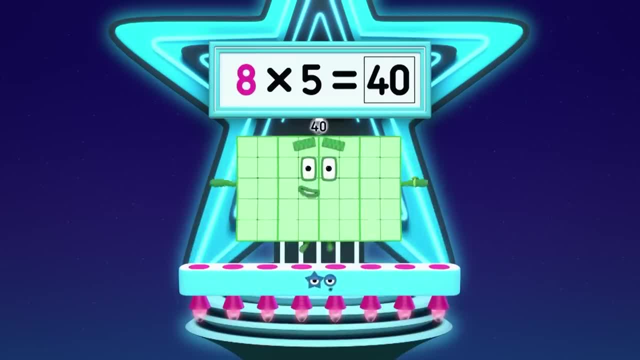 you know who we are. you know who we are. seven fives are thirty-five. eight fives. seven fives are thirty-five. eight fives, seven fives are thirty-five. eight fives are. forty are forty, are forty. forty five. here's the next big. forty five, here's the next big. 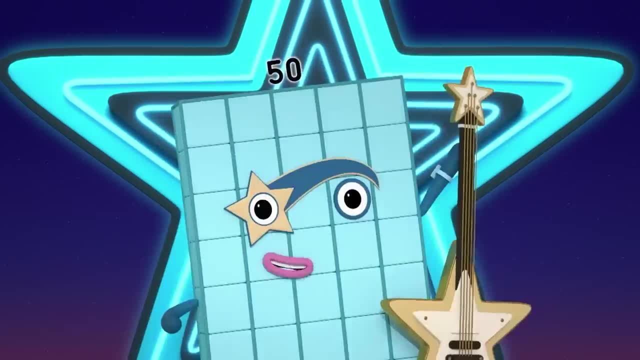 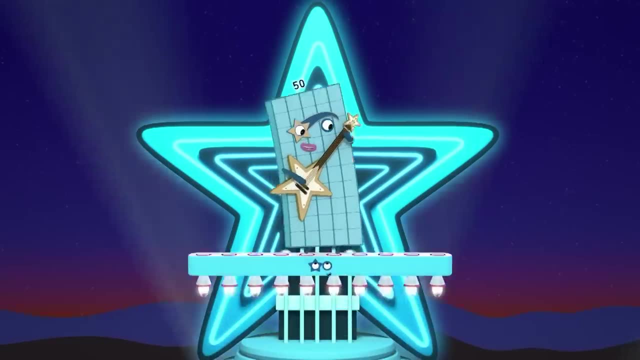 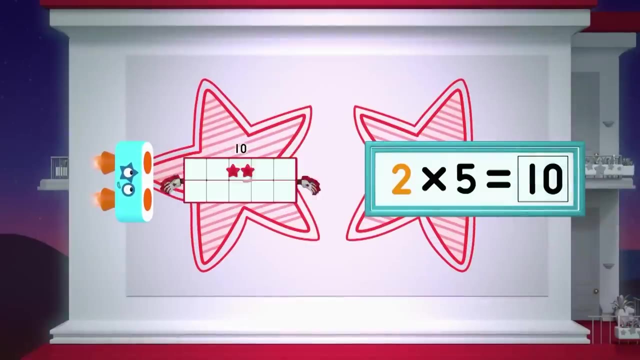 forty five. here's the next big superstar. ten fives are fifty. superstar. ten fives are fifty. superstar. ten fives are fifty. guitar solo, sideways, sideways, sideways. one five is five, two fives are ten. one five is five. two fives are ten. one five is five. two fives are ten. three fives are fifteen. trust me, you'll go. 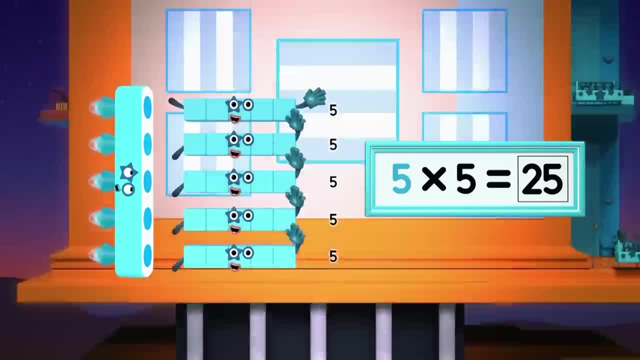 three fives are fifteen. trust me, you'll go. three fives are fifteen. trust me, you'll go far, far far. four fives are twenty five. fives are four. fives are twenty five. fives are twenty five. four fives are twenty five, fives are twenty five. 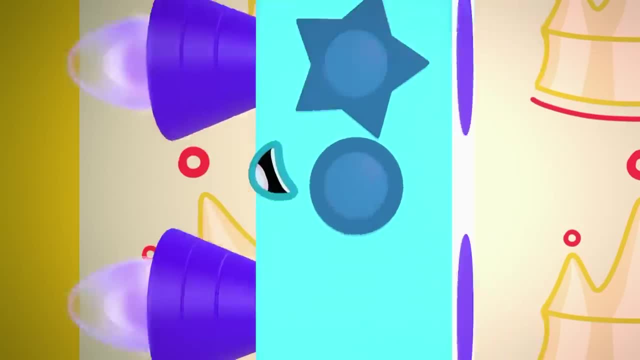 four fives are twenty five. fives are twenty five. six fives are thirty. six fives are thirty. six fives are thirty. you know, six fives are thirty. you know who we are, who we are, who we are. seven, five to thirty-five. eight fives are: 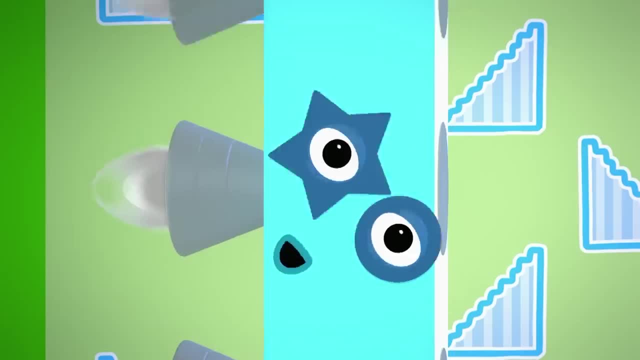 seven, five to thirty-five. eight fives are seven. five to thirty-five. eight fives are forty, forty, forty, nine, five to forty-five- one more time. nine five to forty-five- one more time. nine, five to forty-five: one more time. let's take it to the top. he's the star. 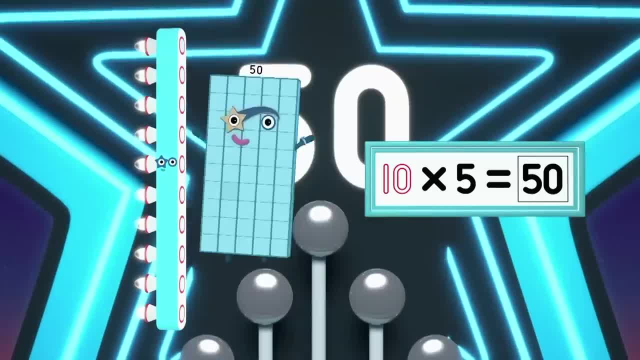 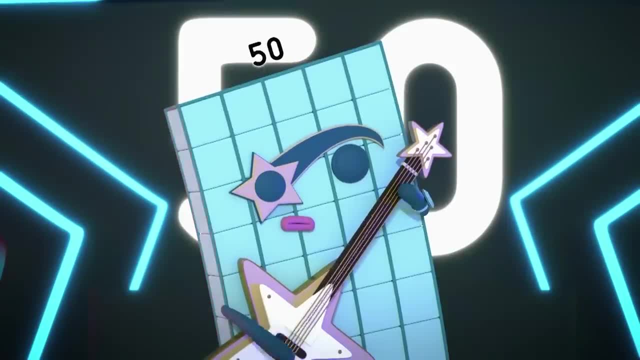 let's take it to the top. he's the star. let's take it to the top. he's the star of the show, of the show, of the show. ten fives are fifty rock and ten fives are fifty rock and ten fives are fifty rock and roll. 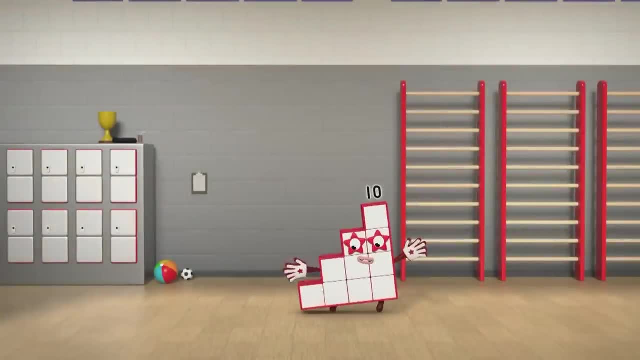 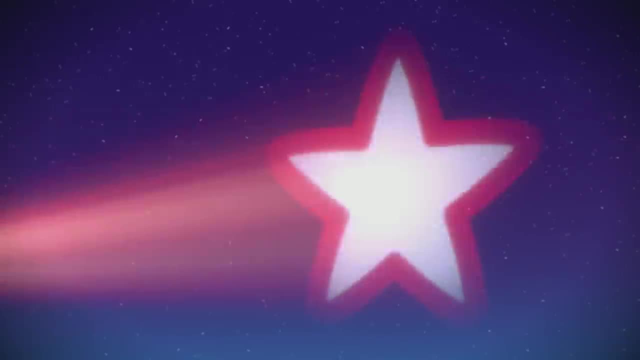 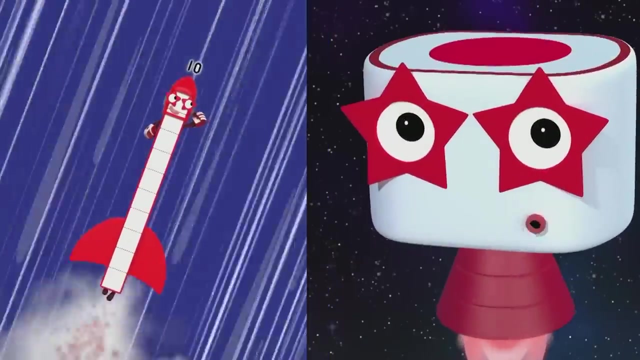 oh yes, oh yes, oh yes. ten, ten, ten, ten. oh yes, ten, ten, ten, ten. oh yes, ten, ten, ten ten. heroes with zeros. this is the ten times heroes with zeros. this is the ten times heroes with zeros. this is the ten times. table, table, table. rocket rescuers. come as soon as you are. 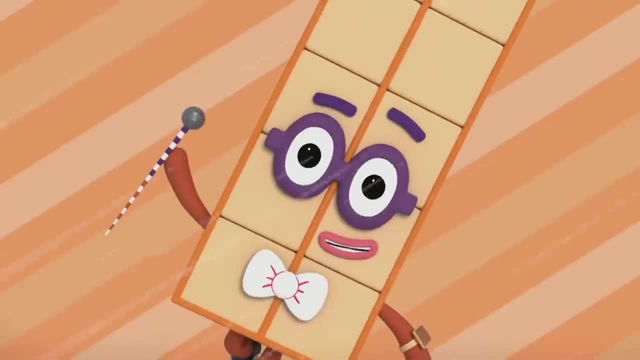 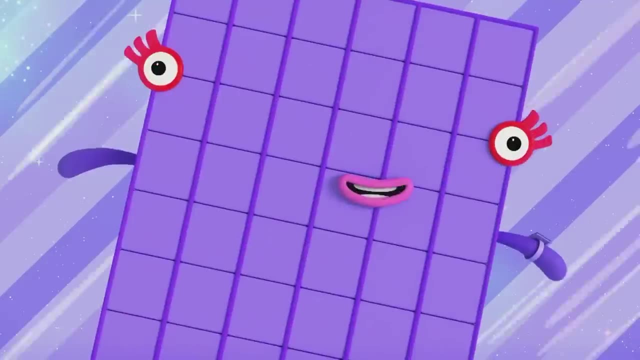 rocket rescuers: come as soon as you are rocket rescuers, come as soon as you are able. able able: 10, 20, 10, 20, 10, 20, 30, 30, 30, 40, 40, 40, 50, 50, 40, 60. 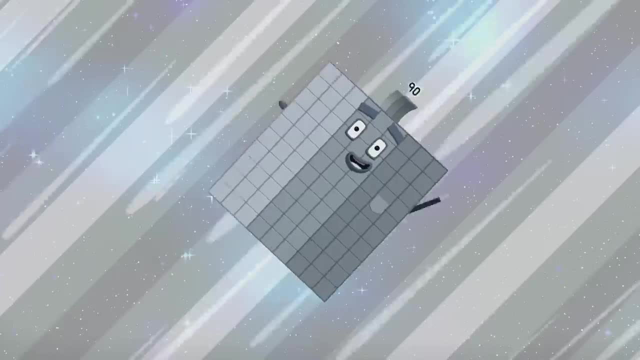 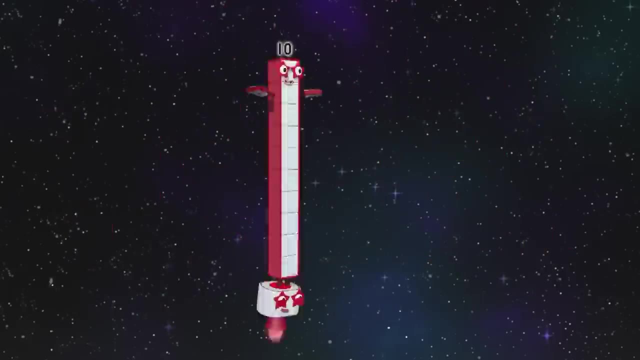 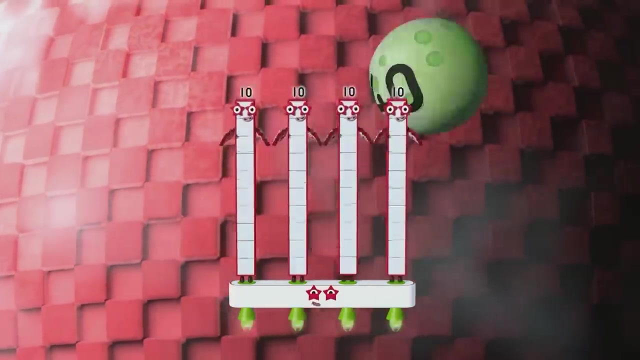 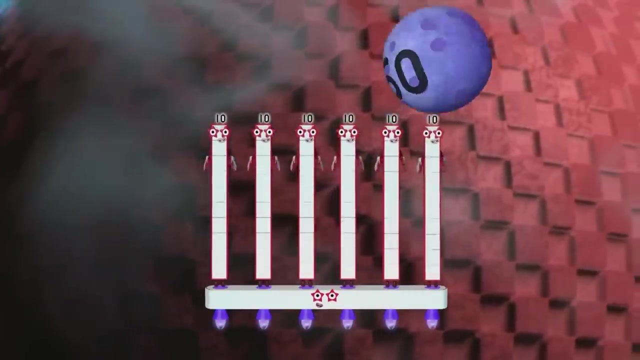 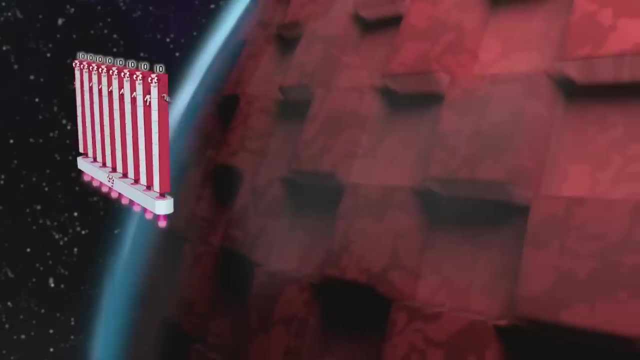 60, 60, 70, 70, 70, 70, 70, 80, 80, 80, 80, 80, 80, 80, 90, 80, 80, 90, 90, and ten tens are 100 heroes with. and ten tens are 100 heroes with. 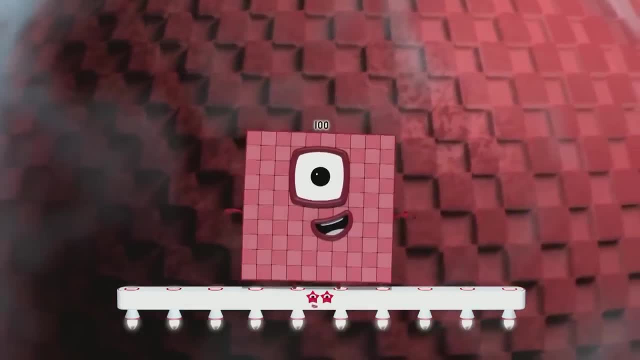 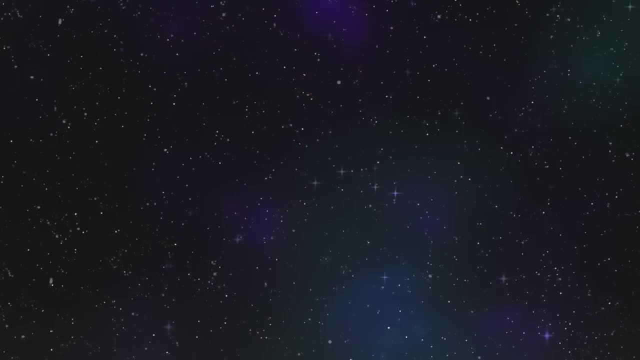 and ten tens are 100 heroes with zeros. zeros and ten tens are 100 heroes with zeros. heroes with zeros, heroes with zeros. 10 is the original, she'll get us underway. 10 is the original, she'll get us underway. 10 is the original, she'll get us underway. rocket to the rescue. 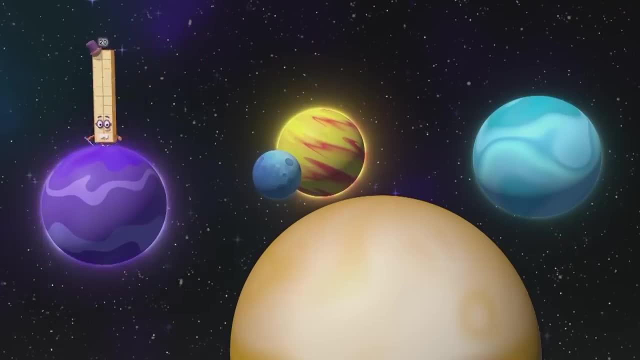 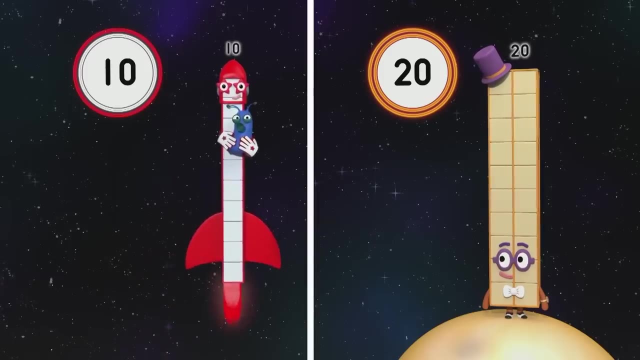 20 has a double boost. he can dance all. 20 has a double boost. he can dance all. 20 has a double boost. he can dance all day interterrestrial tango. they know what their zeros. they know what their zeros. they know what their zeros for. 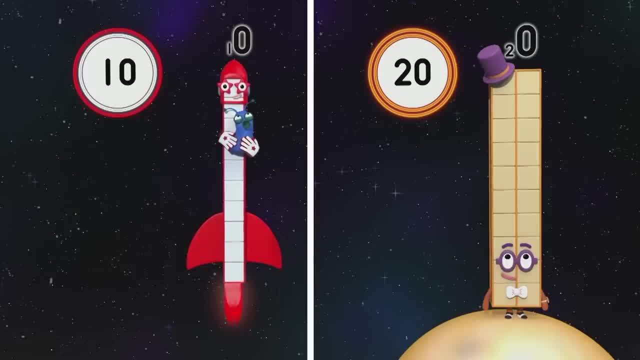 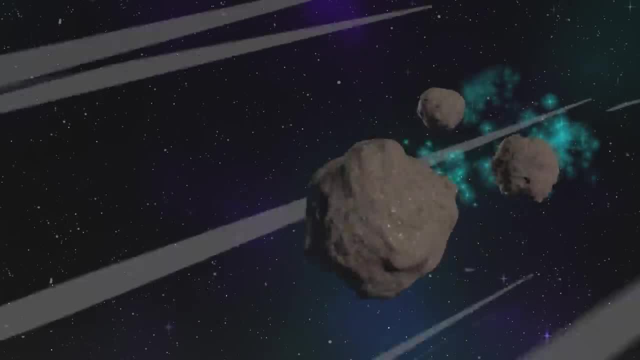 they know what their zeros for. they know what their zeros for: one ten, two tens and nothing more. one ten, two tens and nothing more. one ten, two tens and nothing more. 30 juggles asteroids: you ain't seen nothing yet. the greatest show in space. 30 juggles asteroids: you ain't seen nothing yet. the greatest show in space. 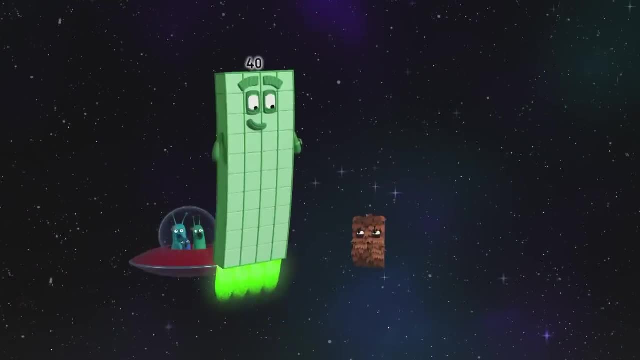 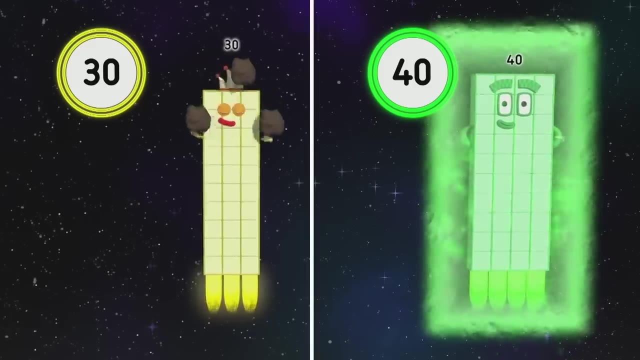 30 juggles asteroids. you ain't seen nothing yet. the greatest show in space: 40 is a rectangle with an oblong. 40 is a rectangle with an oblong. 40 is a rectangle with an oblong, pet galactic oblong. they know what their zeros for. 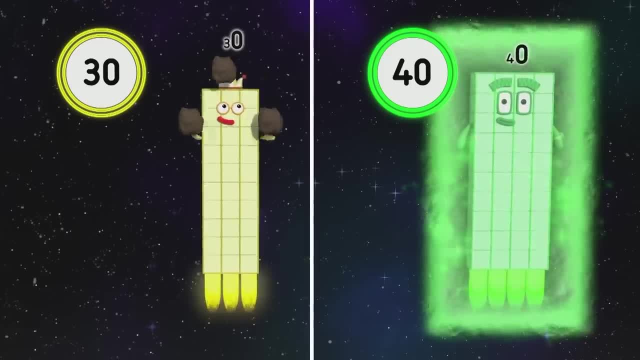 they know what their zeros for. they know what their zeros for three tens, four tens and three tens, four tens. and they know what their zeros for three tens, four tens and nothing more. heroes, nothing more heroes, nothing more heroes. 50 is a superstar. 50 is a superstar. 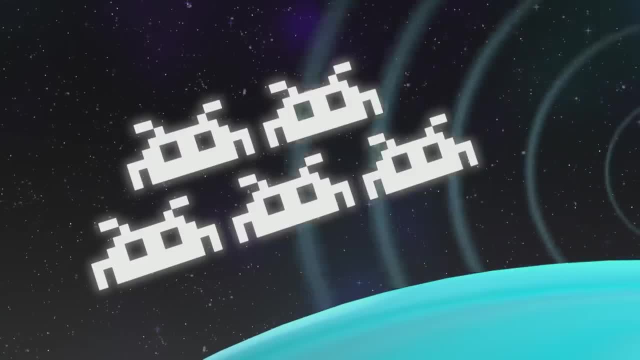 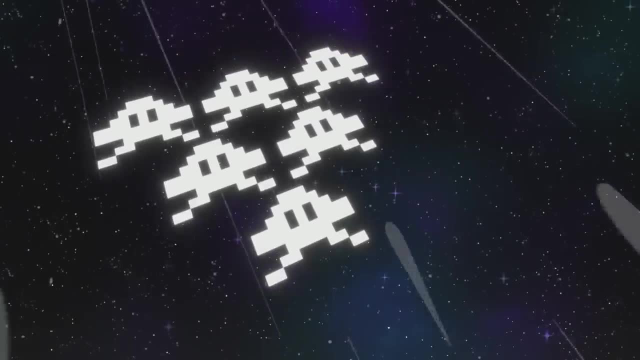 50 is a superstar. who works the satellites interstellar? who works the satellites interstellar? who works the satellites interstellar? overdrive, overdrive, overdrive. 60 is a super gamer. 60 is a super gamer. 60 is a super gamer. she can light the lights. galactic game. 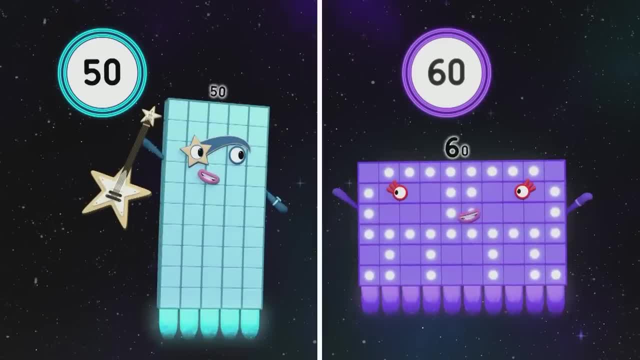 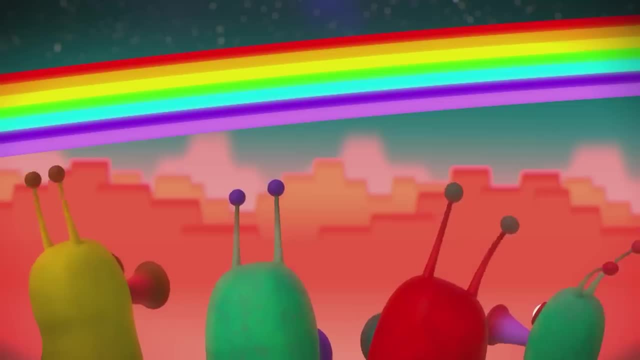 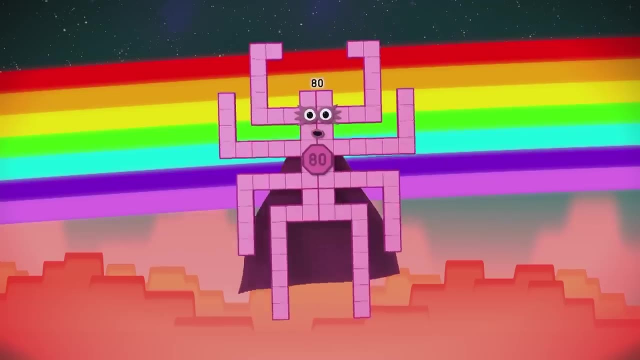 70 has luck times. 10 launching from the duck space rainbow, from the duck space rainbow, from the duck space rainbow. katie needs no luck at all, he's super katie needs no luck at all. he's super katie needs no luck at all, he's super octoblocks. 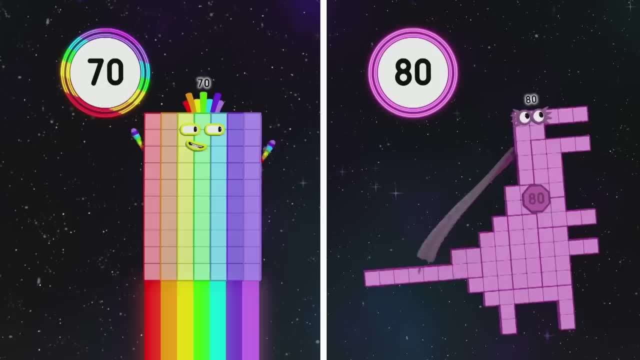 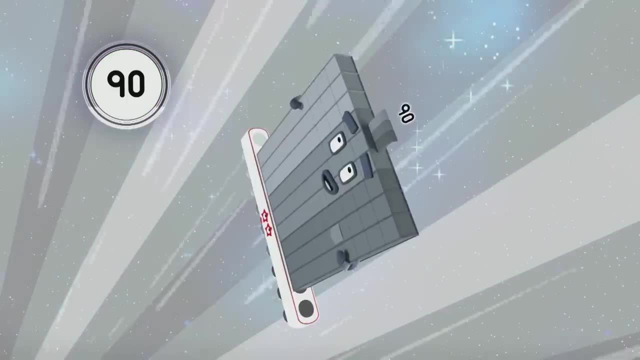 octoblocks, octoblocks. they know what they're zeros for. they know what they're zeros for. they know what they're zeros for: seven, tens, eight, tens and nothing more. seven tens, eight, tens and nothing more. seven tens, eight, tens and nothing more. heroes with zeros. 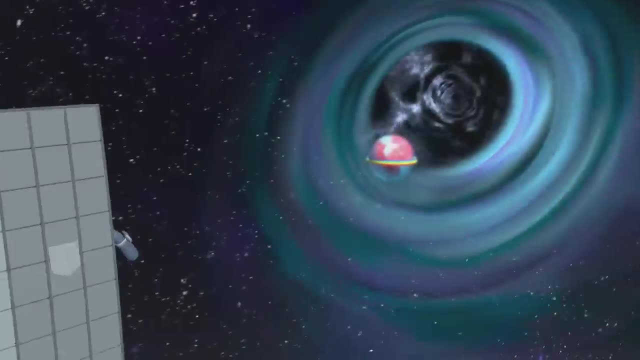 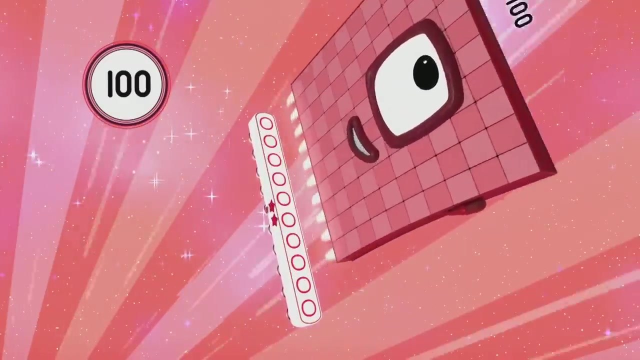 heroes with zeros. heroes with zeros: nighty knows a trick or two. he will. nighty knows a trick or two, he will. nighty knows a trick or two. he will heed the call: abracadabra, abracadabra, abracadabra, abracadabra. and now let's meet 100. 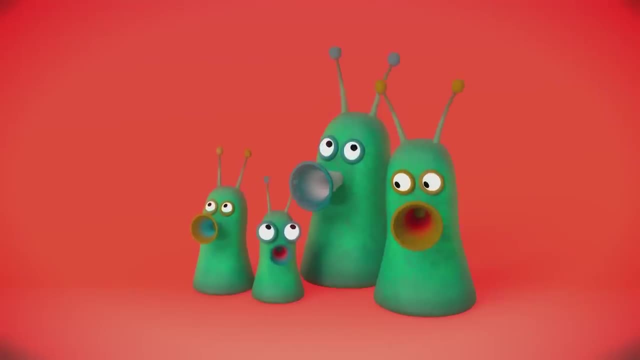 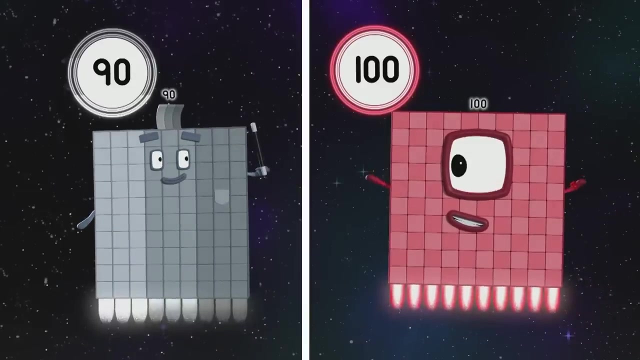 and now let's meet 100. and now let's meet 100, the greatest of them all, the greatest of them all, the greatest of them all. hero with two zeros. hero with two zeros. hero with two zeros. nine tens, ten tens heroes with zeros. nine tens, ten tens heroes with zeros. 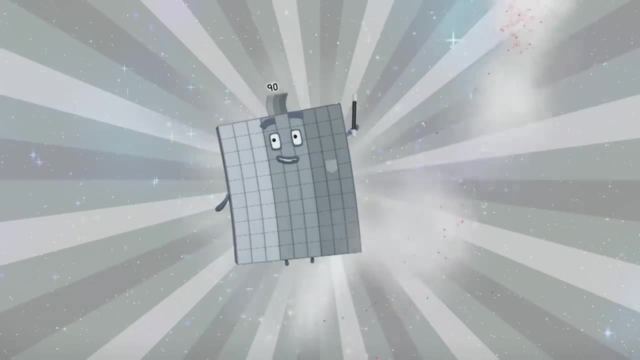 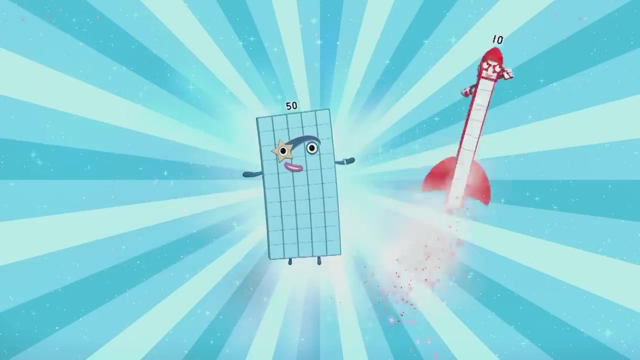 nine tens ten tens heroes with zeros: 100, 100, 100, 90, 90, 90, 80, 80, 80, 70, 70, 70, 60, 60, 60, 60, 60, 50, 50, 50, 50, 50, 40. 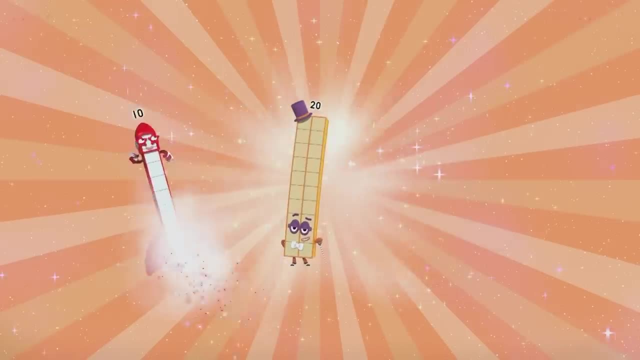 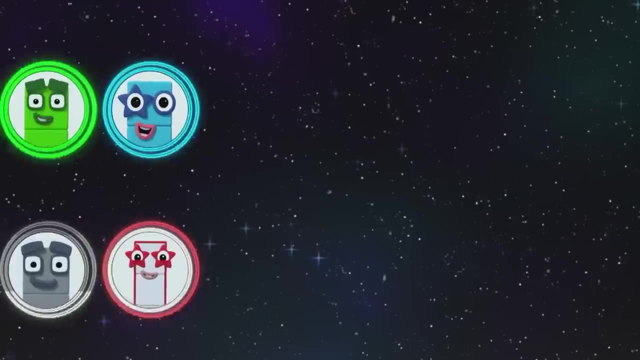 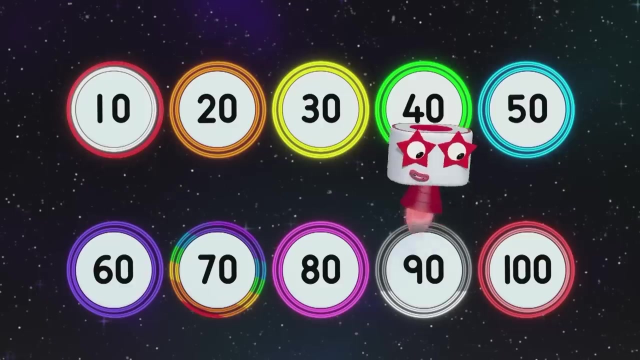 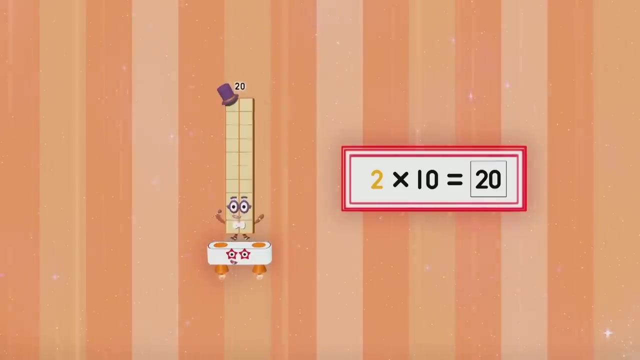 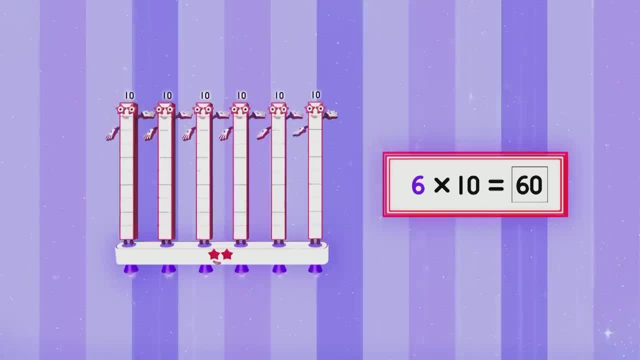 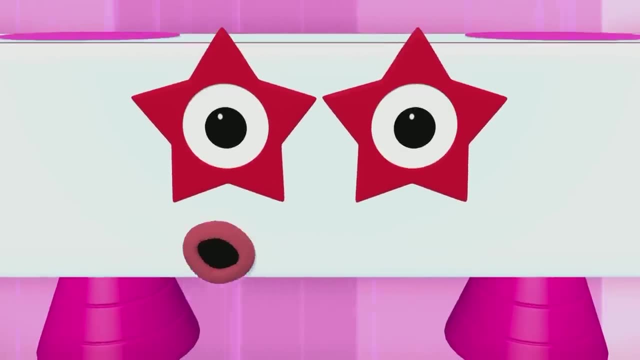 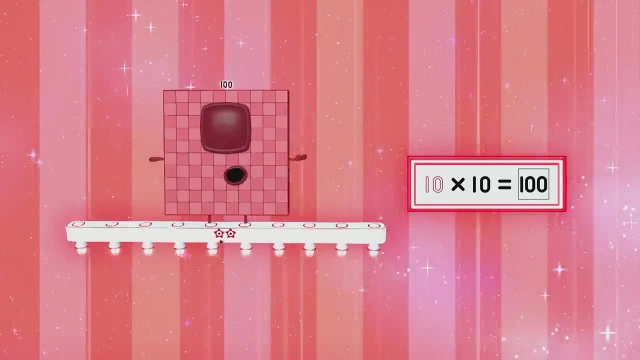 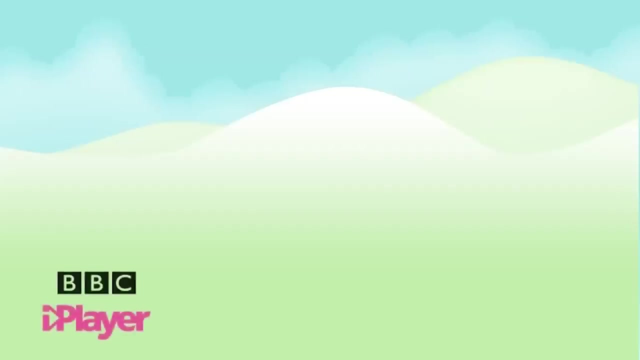